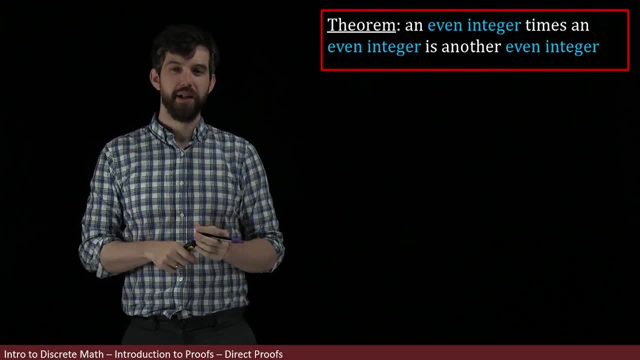 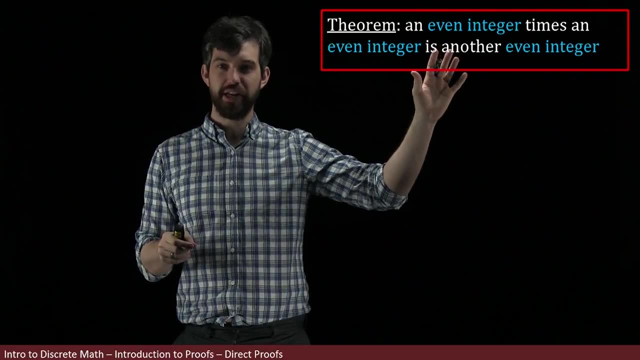 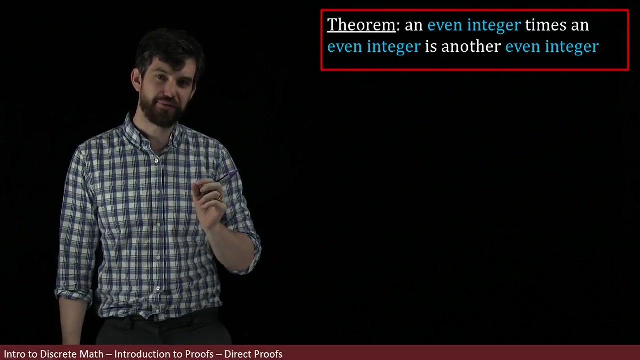 as well as everything else sort of filler and connective tissue. But the main word that we need a definition for is the idea of an even integer, And we might be able to come up with an even integer definition relatively quickly but for more complicated theorems, focusing very precisely on what it means for each of these. 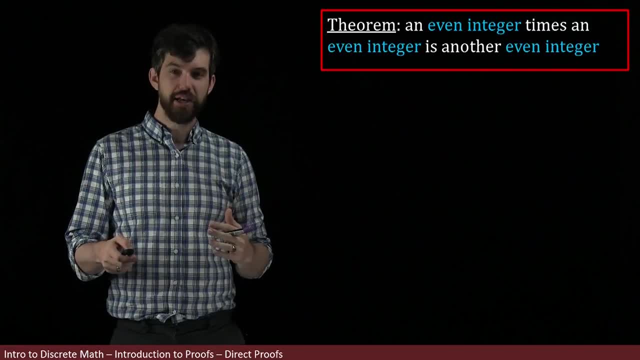 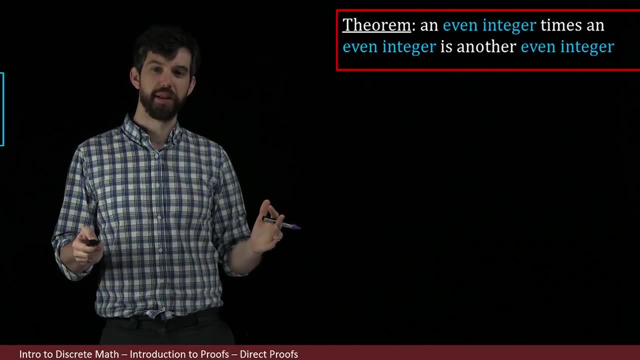 words is going to be an almost necessary first step. So let's go back and, before we even get to this theorem at all, let's investigate the idea of an even integer. So my sort of informal definition of an even integer is that it's an even integer if it. 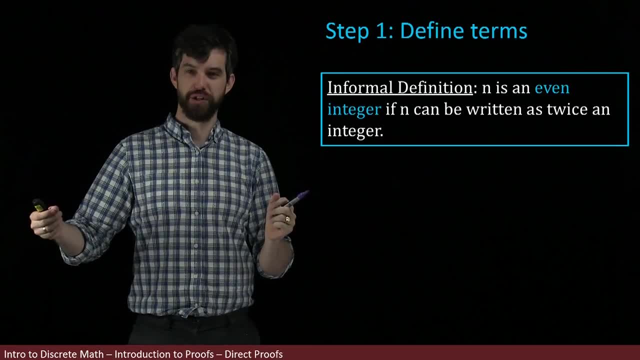 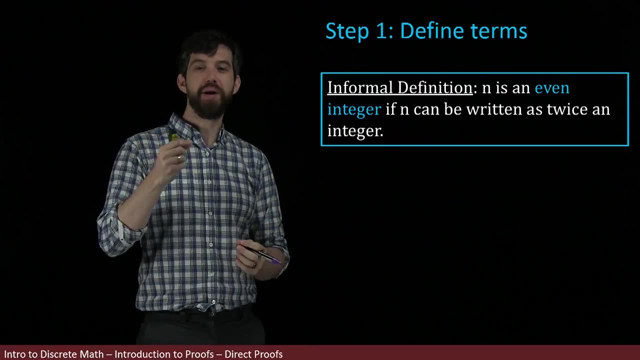 can be written as twice some other integer. So for example, like six is twice three, or twelve is twice six and so on. So if I can write my integer as twice some other integer. But I want to be even a little bit more mathematically. 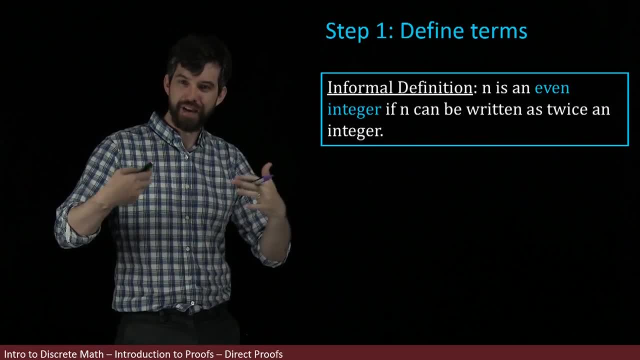 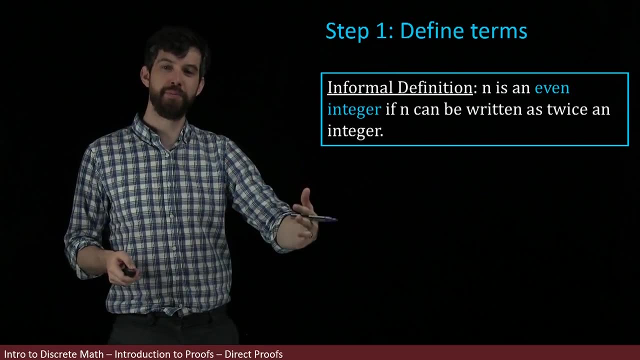 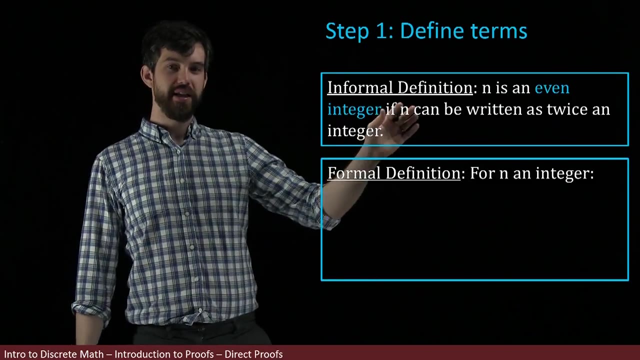 precise with this particular definition. I want to use all of the fancy terminology that we've been developing in this course that has a lot of precision to it and will be very amenable to manipulating as we go on in our proof. So I want to come up with a formal definition Now. notice that in my informal definition, 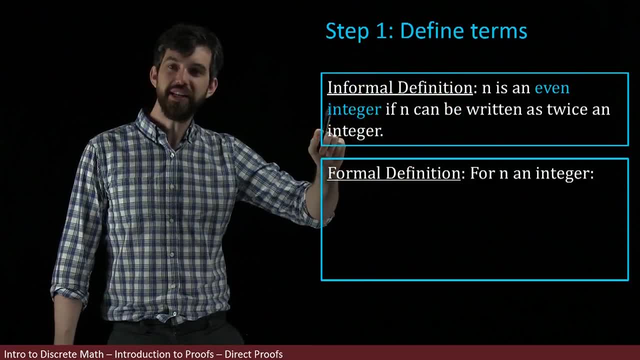 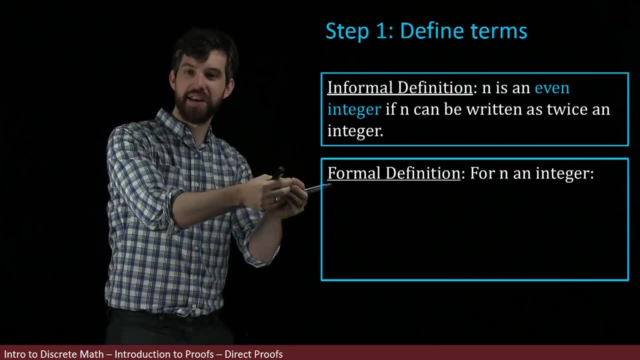 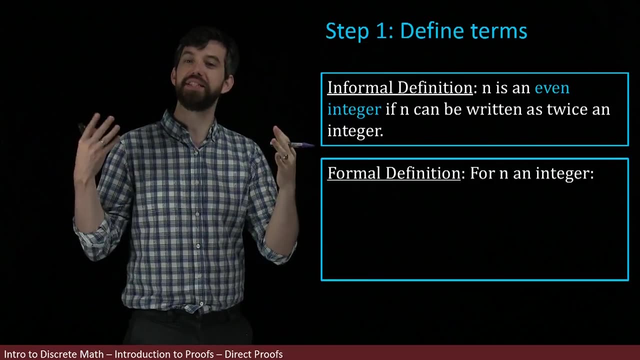 what I have is n is an even integer. if there's an existence claim snuck in here, If there exists some number such that twice that number is what I began with. So that's what I want to note is that inside of this informal definition is an existence claim. You are claiming it. 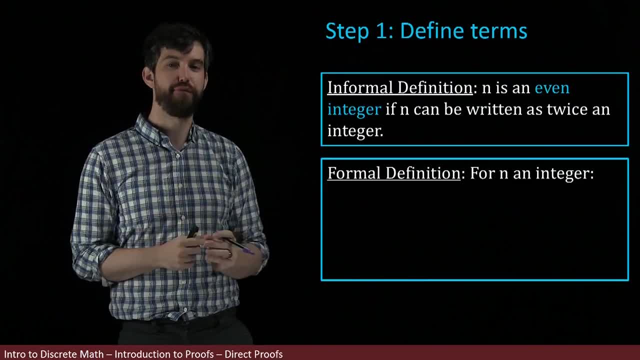 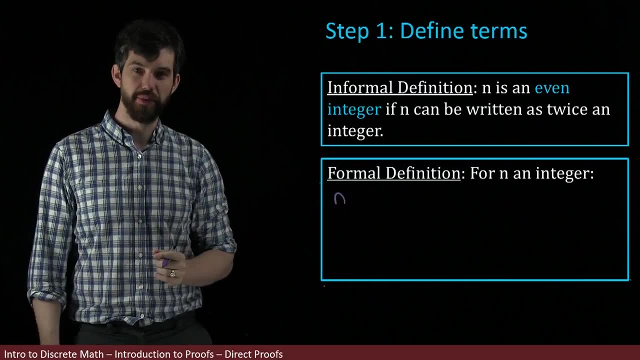 can be written in some way, and I want to express that in my formal definition. So here's how I'm going to translate it: I'm going to say that n, that's my integer under description, And I'm going to say that n is an even integer. That's what I'm trying. 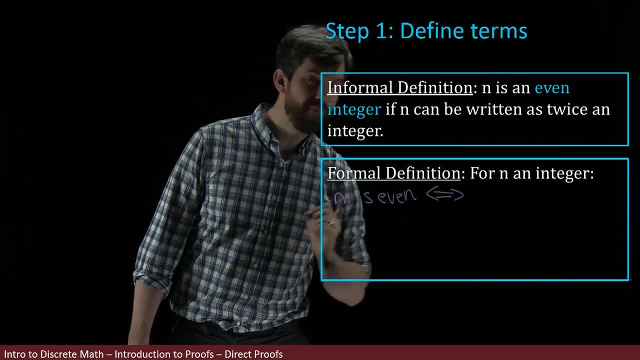 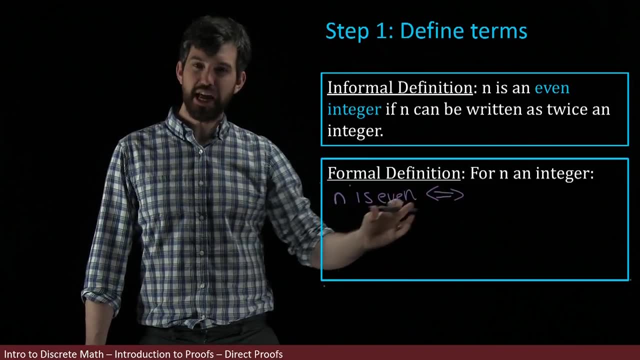 to claim. And note that I'm now going to put the biconditional symbol here, And the reason I write this biconditional arrow here is that all of these definitions work two different ways. The definition of even is going to be the stuff I'm going to write down and then 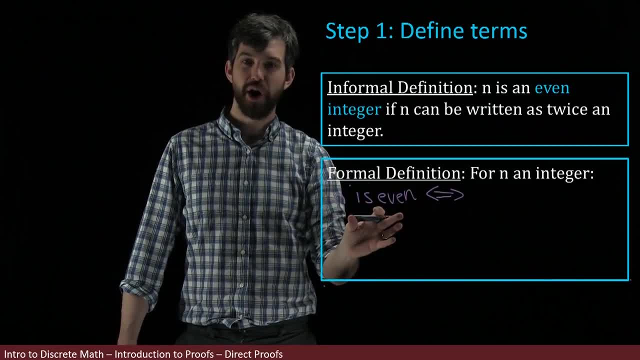 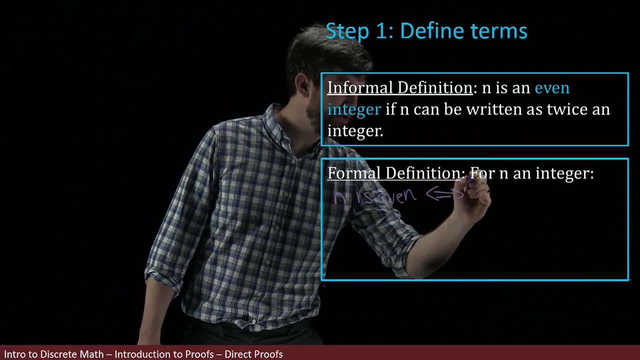 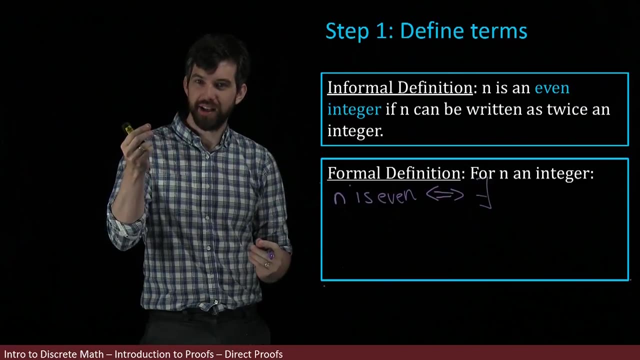 if you have the stuff I'm going to write down, you're going to get even. So all definitions are if, and only if, I have n even. And what do I want to claim? I want to claim that there exists something, There exists some other integer such that your n can be written as twice this integer. 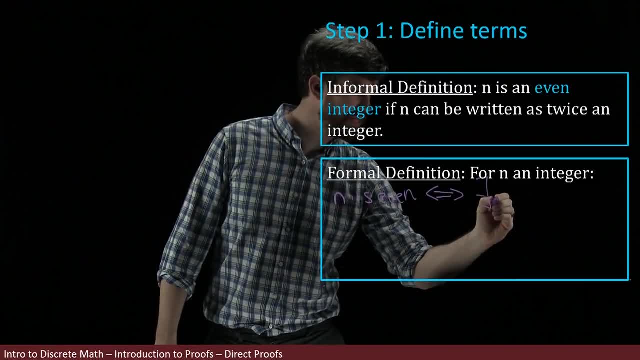 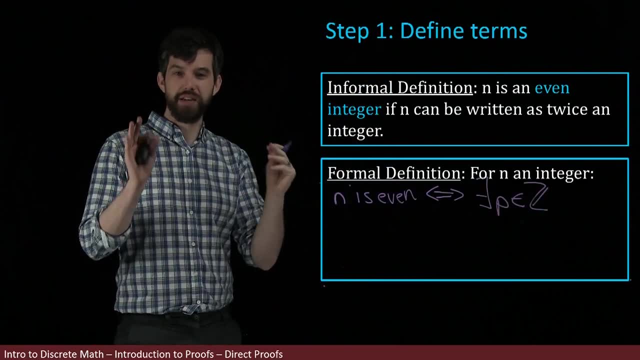 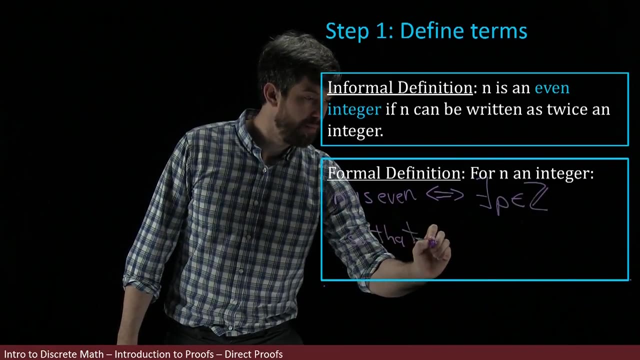 that we're describing, So I'm going to get a given name for it. I'm going to say that there exists a p And I'm going to write it like this: There exists a p inside of the integer, So there exists some other integer, And then so that 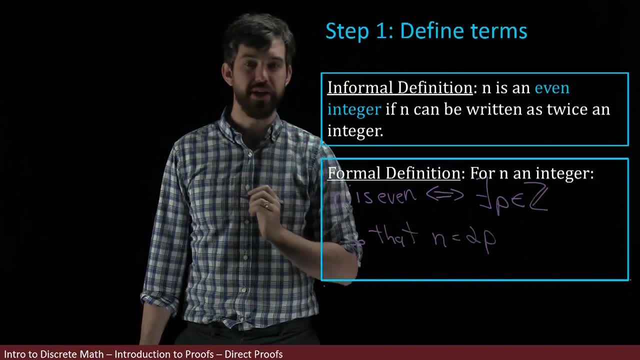 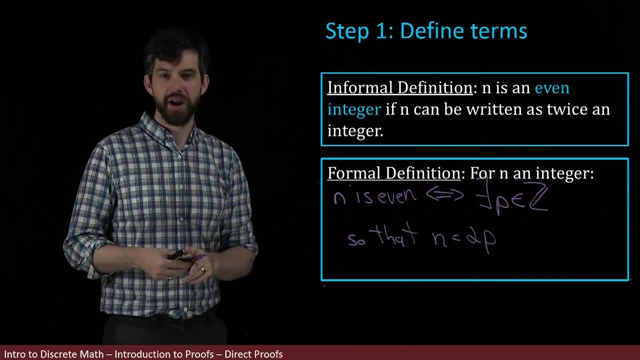 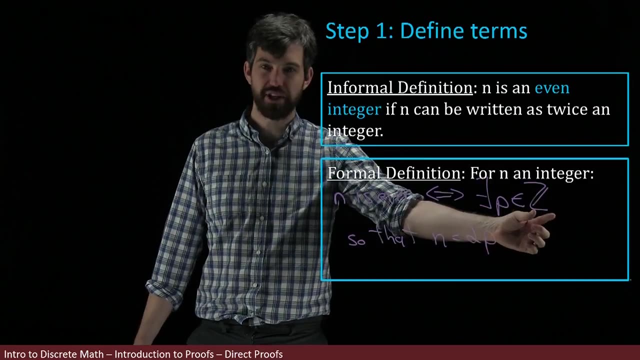 My n is equal to twice that other integer p, And that is going to be my formal definition. Note that you have some leeway here. I chose to use the backwards e for there exists, and the e symbol here for element of, and the integers, to have this sort of real shorthand for the 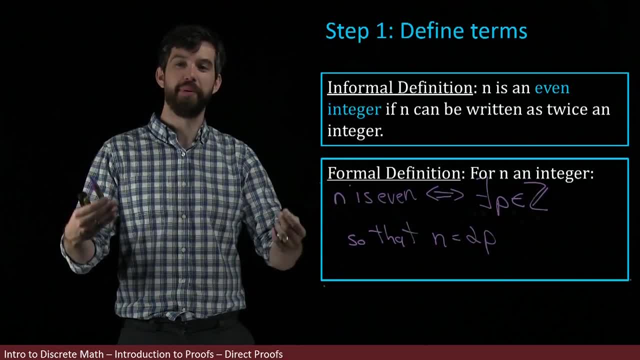 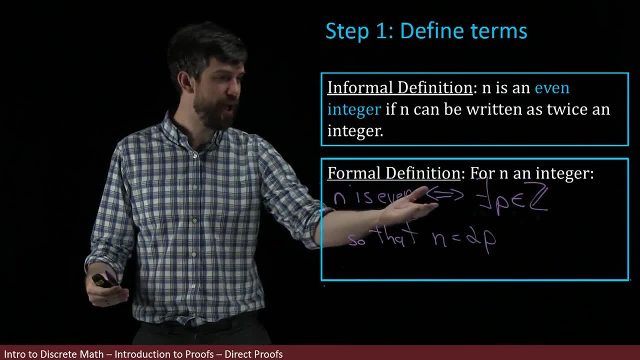 larger English phrase. there exists a number p in the integers. If you prefer to write down the larger English phrase, there exists a p inside of the integer. you're going to have a p in the integers instead of my mathematical shorthand. I have no objection to that. I. 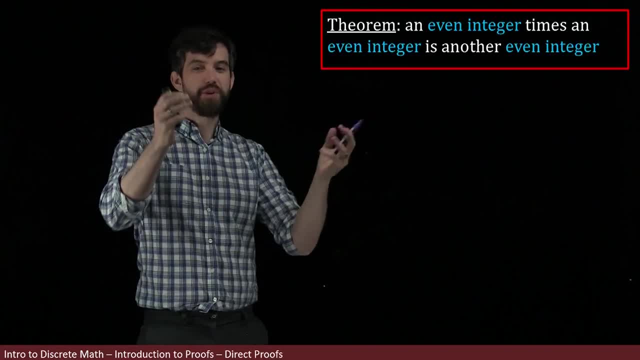 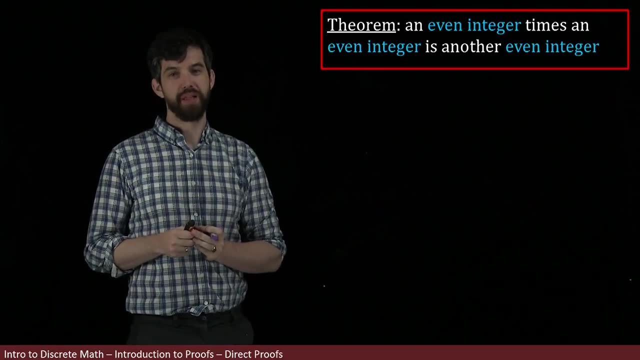 just like being efficient on the board. All right, So back to our theorem. So now we know what an even integer is And if we need to going forward, we can always go back and recall that. But my next point is that 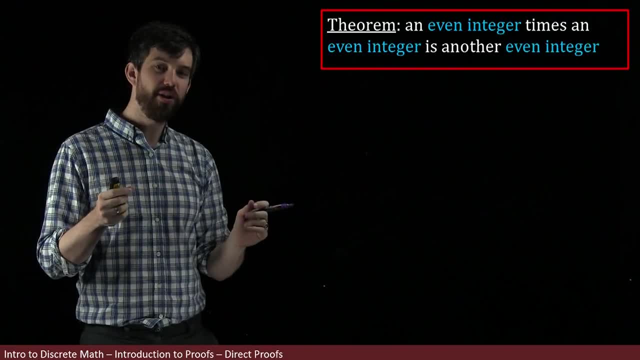 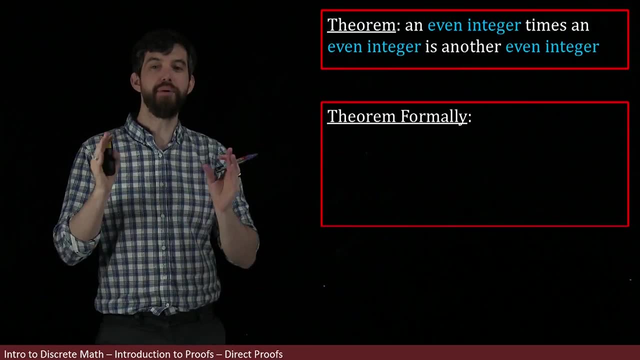 my theorem that I have written down here is written a little bit informally And I want to clean it up a little bit. I want to say it in a little bit more of a precise manner. So I want to describe what my theorem says formally. 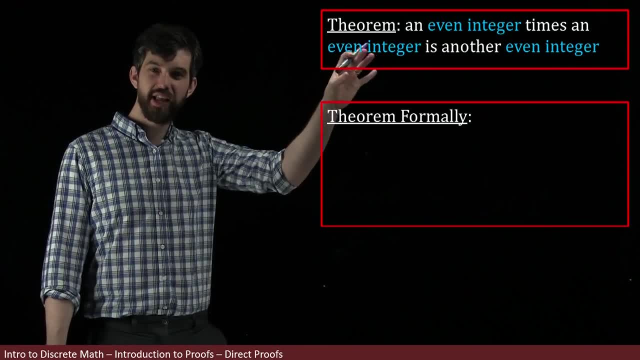 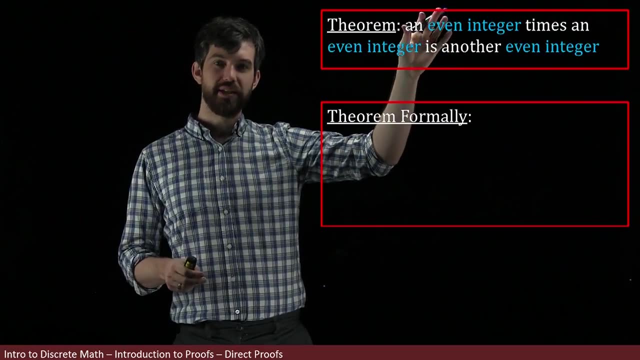 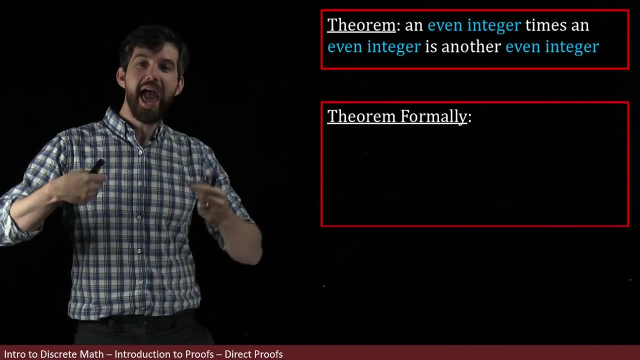 The first thing I want you to note is that there's sort of a hidden universal in my informal presentation of this theorem. It says: an even integer times an even integer is another even integer, But implicit in the way I phrase this is the claim every single time I find. 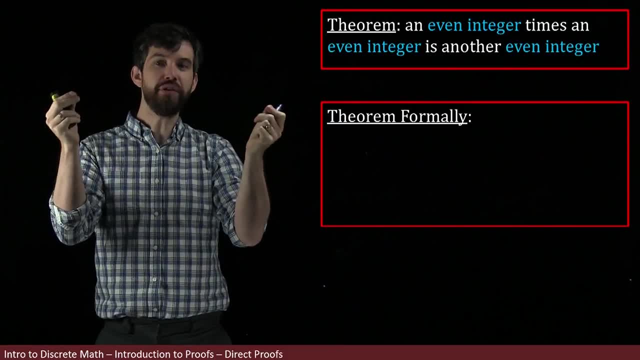 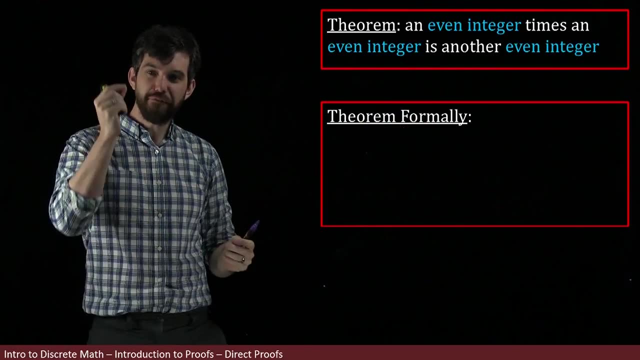 those pairs of integers that are both even every single time, then their product is going to be an integer. So hidden inside of this is an even integer, And I want you to notice that there's a little bit of a for all claim, And so I'm going to write that down. first I'm going to claim. 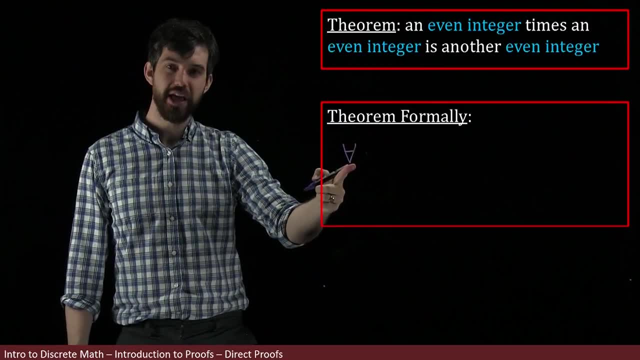 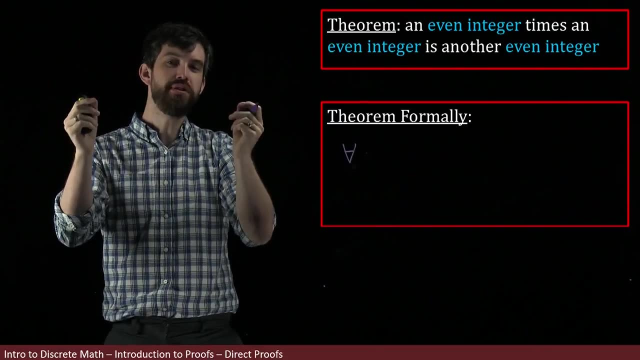 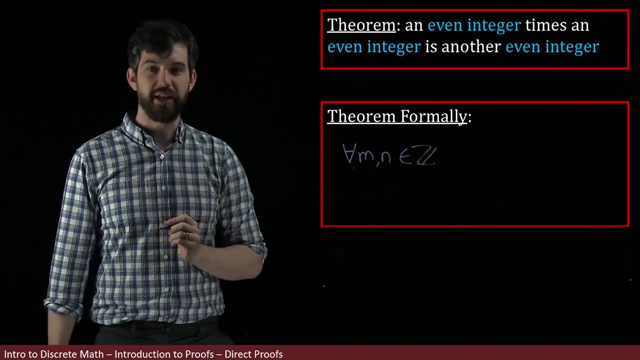 that for all my upside down a for every- and notice it's an- all claim about two different numbers. It's every time I have two different numbers that are even. So for all m and n, they're going to begin as just generic integers. Then I'm going to have that if my m and n 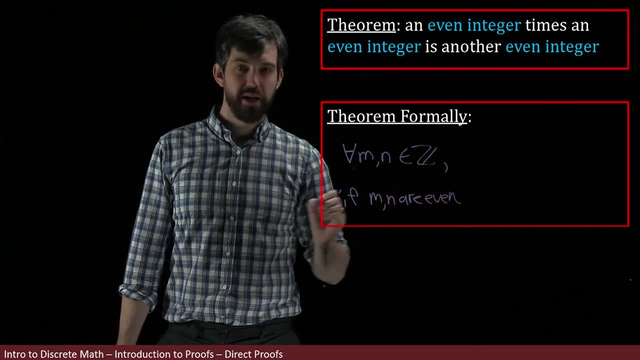 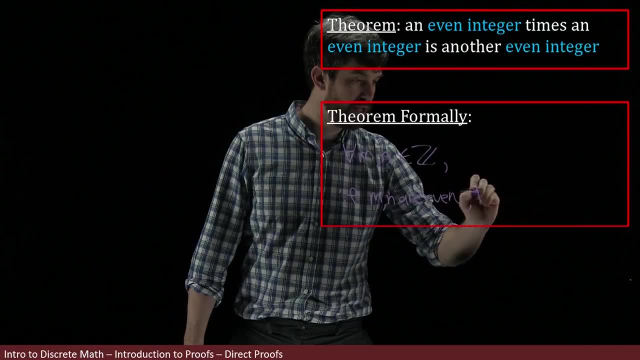 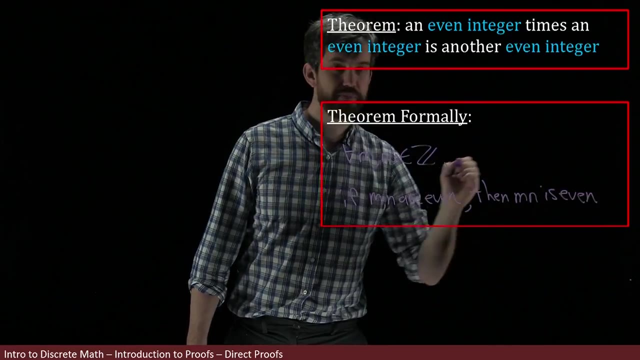 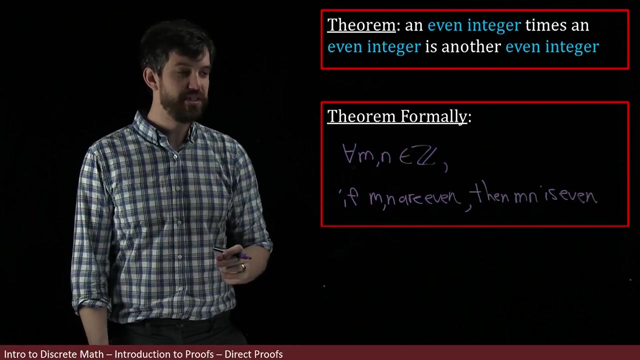 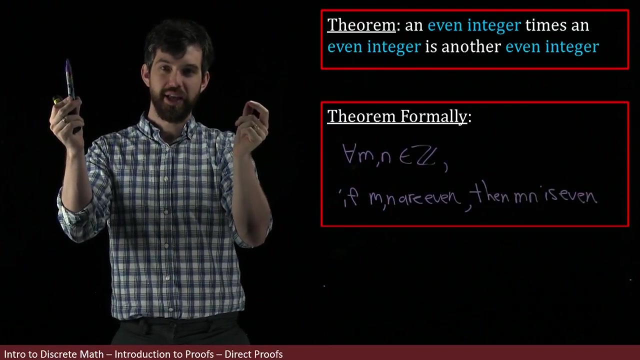 are even, That this is going to lead me to conclude that their product is going to be even as well. Then the product m times n is also going to be even. So the key thing in my formal statement of my theorem here is to note that it says: for every time I take a pair of integers, 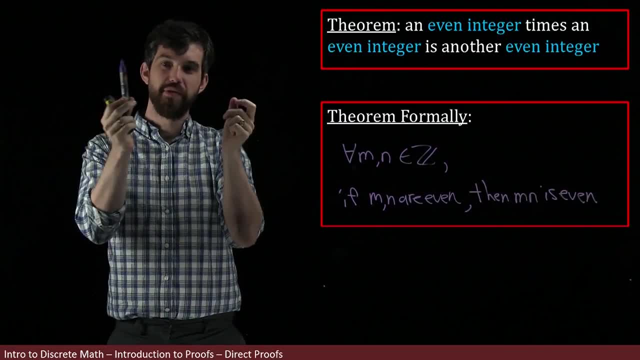 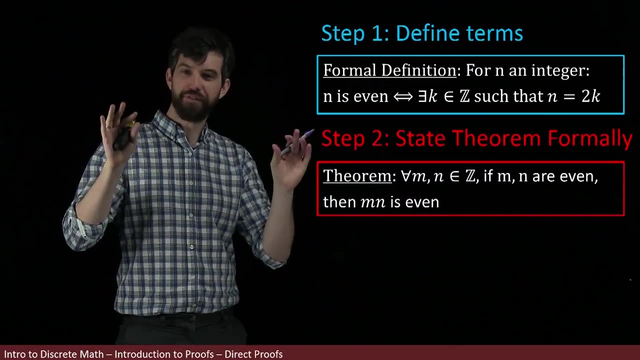 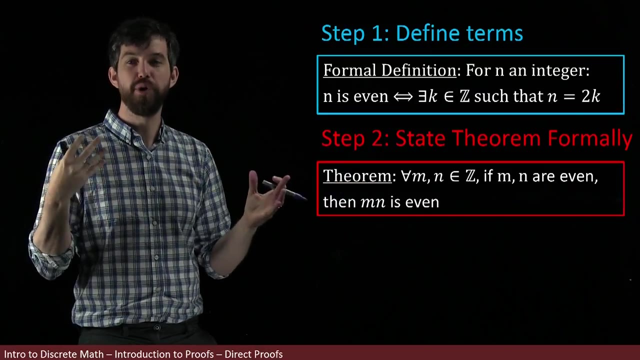 if those pairs of integers that I get are both even, then their product is even as well. All right, So what we've done so far was, step one, we formally defined the different terms in our theorem, And then step two, we took our theorem and we formally wrote it with. 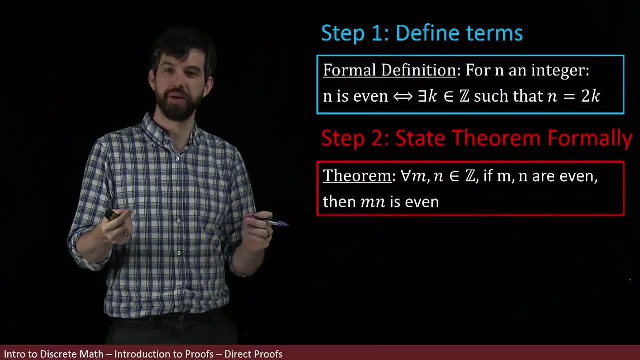 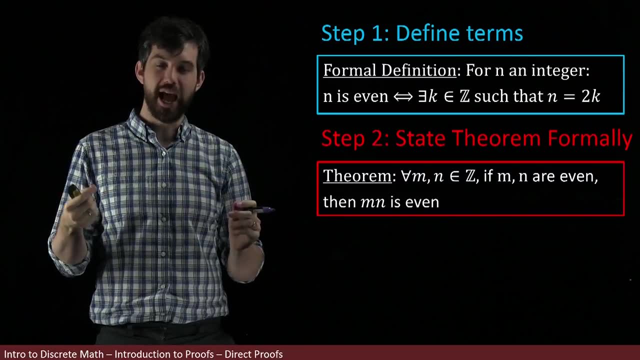 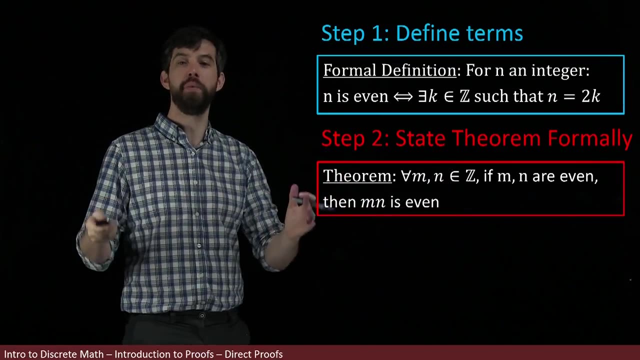 all of our notational shorthands of the for alls but, most importantly, have formally written it in this very precise way that is going to be amenable to manipulating and deducing our theorem. I also want to note that this theorem that we've stated here is in a very common form. 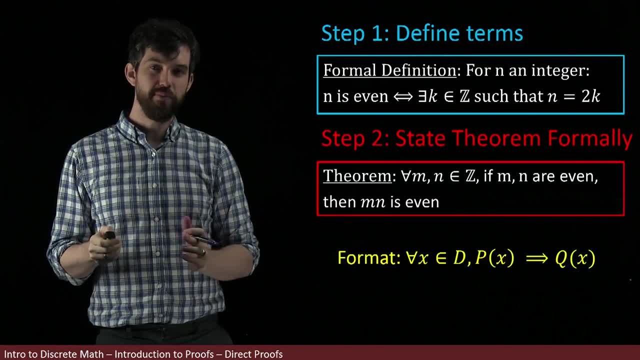 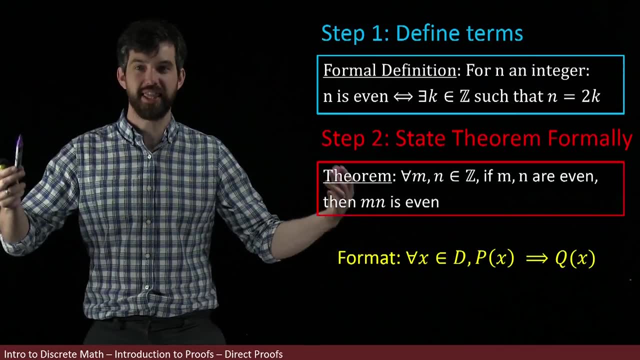 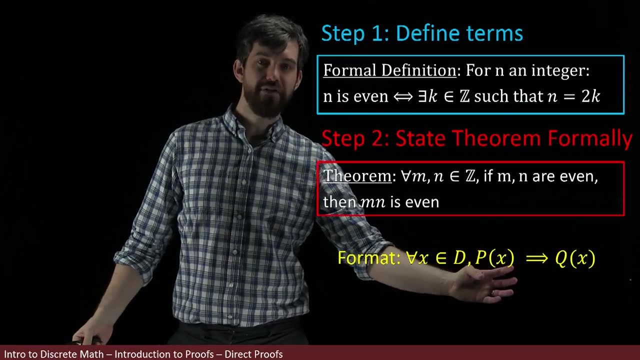 that a large swath of theorems are going to be. In particular, the format of it effectively is: for all things in some domain. In this particular case, the things were pairs of numbers, both in the integers, But for all things in some domain if you have an initial. 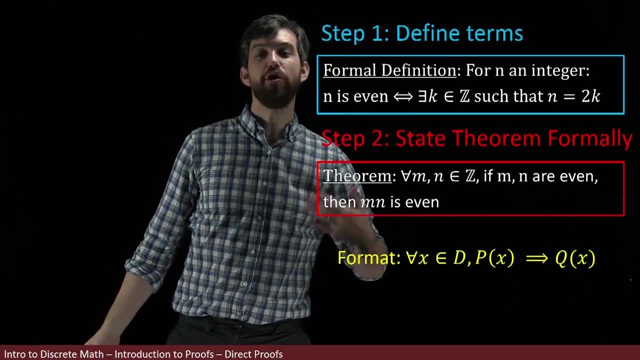 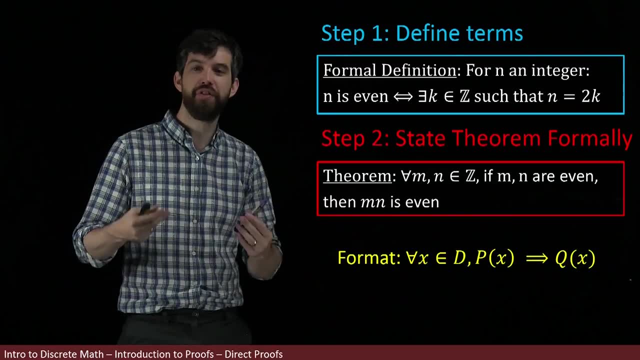 property they're even. then you get some other property, in this case that they're part of, They're products even as well. So this format that we have for stating a theorem is going to be one of the major classes of how theorems are going to be presented. Of course, the domain and the initial predicate. 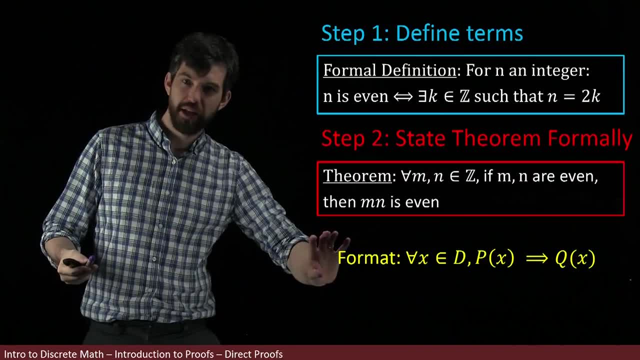 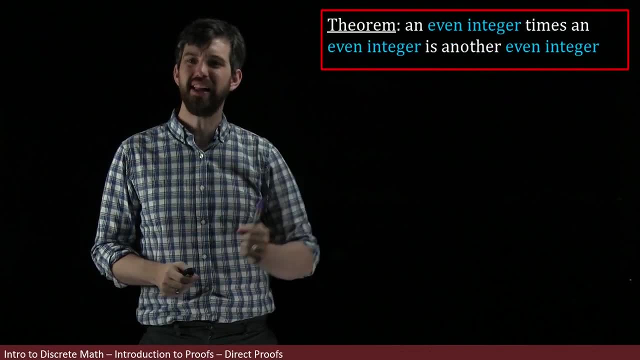 and the final predicate. all of those are going to change from theorem to theorem, But this logical structure is pretty common, All right. So what's next? So let's go back to our theorem, And I'm going to leave it actually in its colloquial form up here. I can bring in its formal definition when and 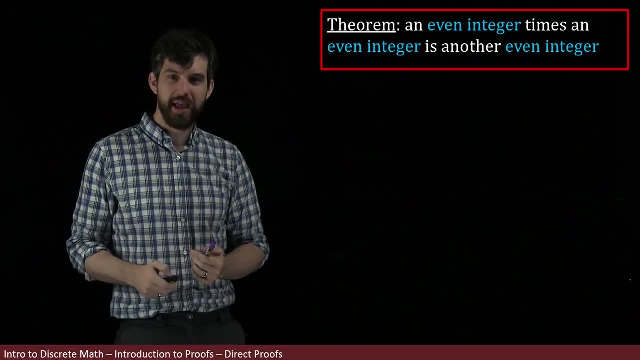 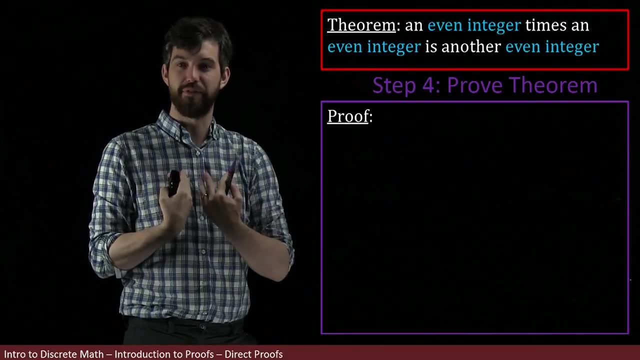 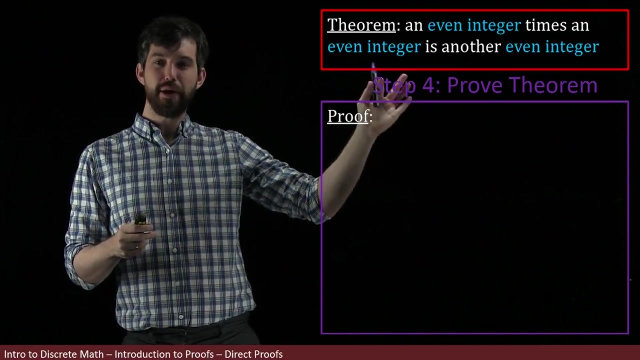 if I need it, Yup, in this convenient way, And remember, what we want to do is: we want to write down some formal proof of this that is going to convince everybody that, yes, indeed, this theorem is valid. However, notice that I write this as step four, because being able to jump immediately to a crystal clear perfect. 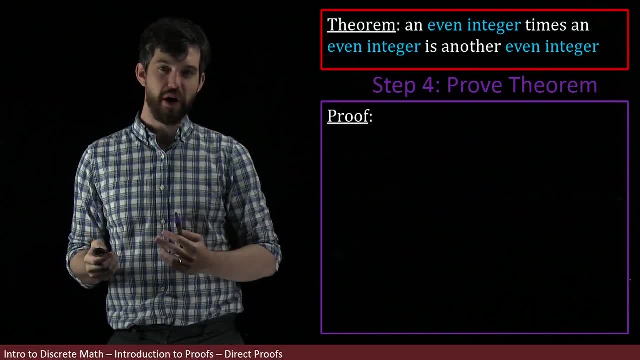 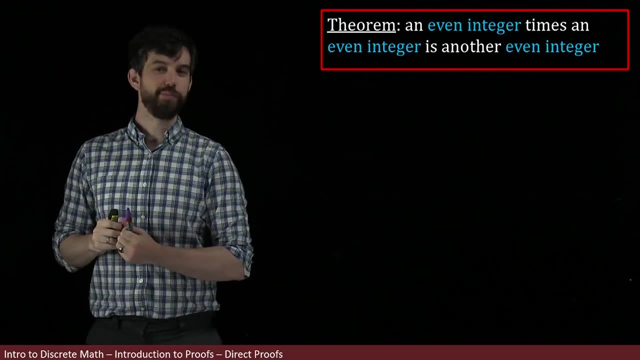 proof is, for most cases, a step too far. In fact, what we want to do is step three, which is the most important step of them all, and that's the step that I like to call playing around, And this is where we try to get some sense for ourselves. not a formal proof, but why do we think this theorem? 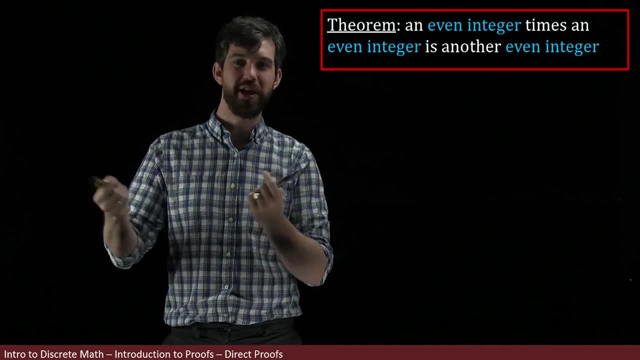 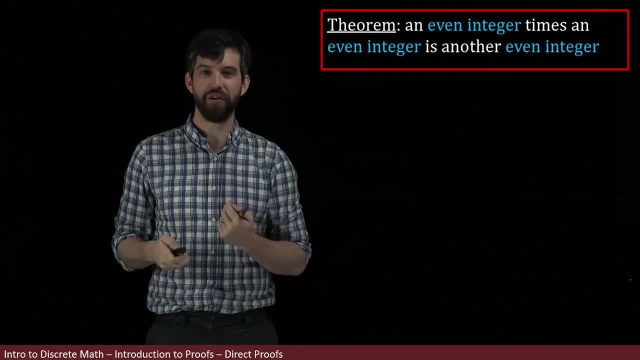 is true. Can I write down a few examples? Can I do some algebraic manipulations? Can I get some sense of why it is that this thing is actually true? And once I have an idea for myself, then I actually can go back and fill it in precisely. So it's important that I'm able to. 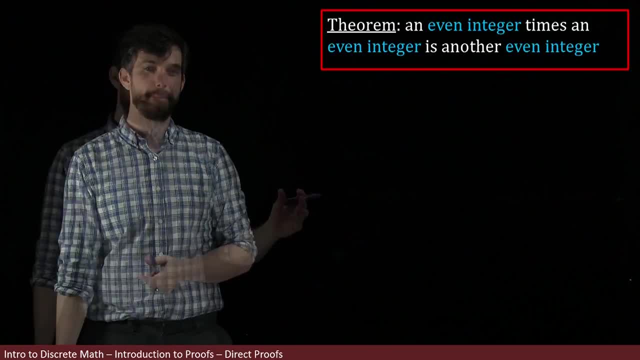 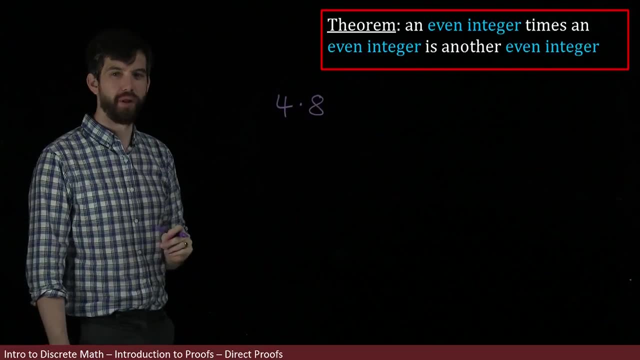 do this. It's important that I'm able to come up with some sort of intuitive idea. All right, so let me just choose a couple different numbers here. How about four times eight, just to sort of get the ball going. And then, if I think about what's going on here, we're going to have 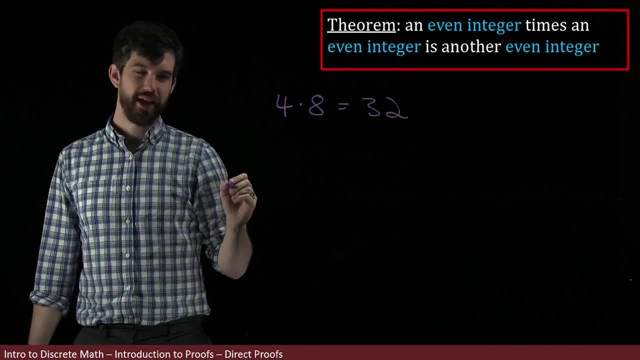 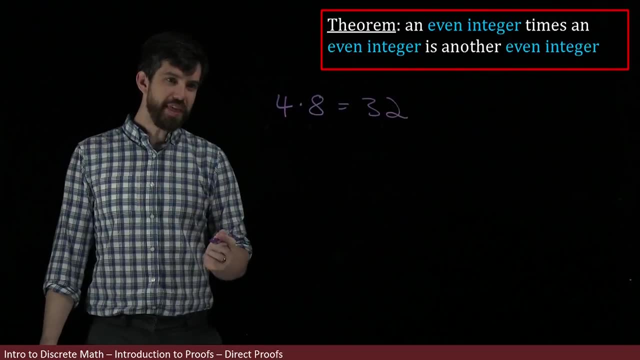 some particular product. In this case it's going to be 32.. And I know that four was even and eight was even and 32 was even. so at least I haven't disproven myself right off the bat. But then, if I think about the four, our definition of an even integer, why do I think four is an even integer? 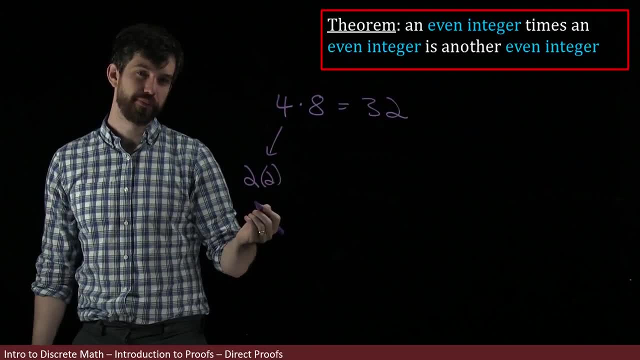 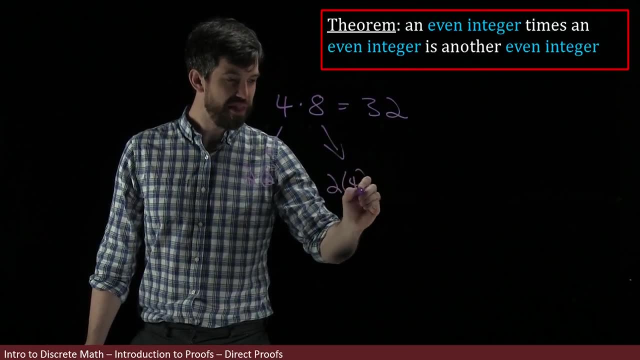 Because it's twice some other number. In this case it's twice two, And the reason why I think that eight here is an even integer is it's twice four. So that's the reason why I think that both four and eight are an even integer, for they're divisible by two, or they can be written in this manner: 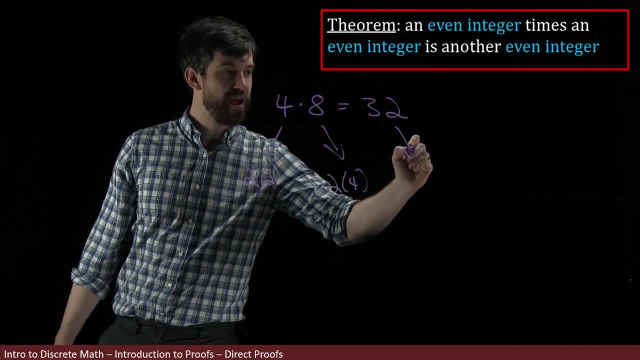 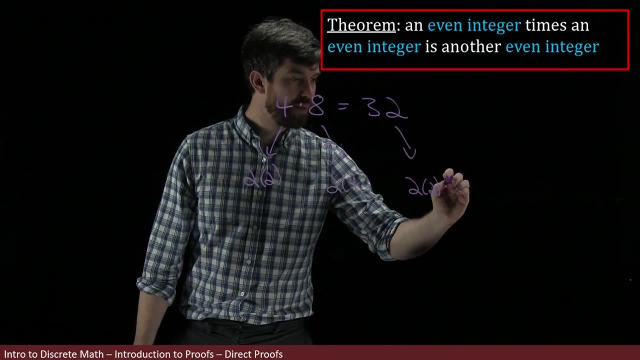 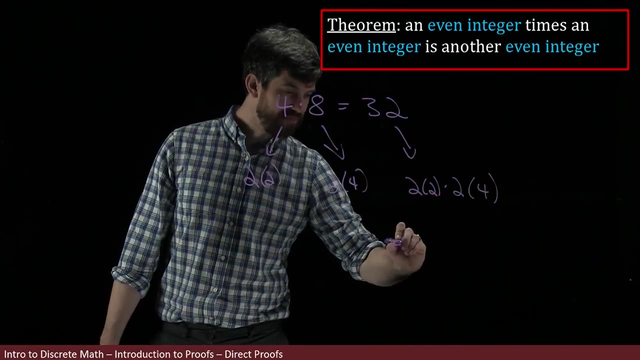 two times this times this. So then, if I go down to my 32, which is the product to these two things, it's like, okay, it's twice two, multiplied by twice four, All right. And then, if I look at this, the way I think about this, you know there's like a two there. 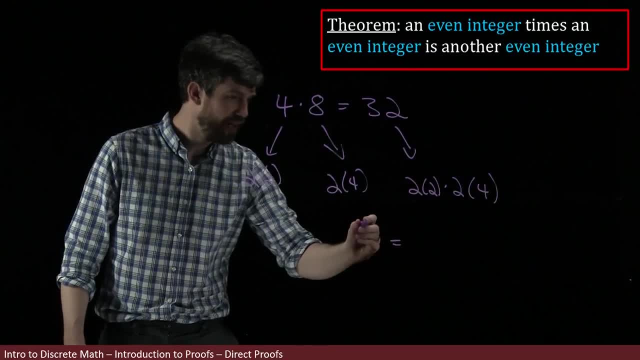 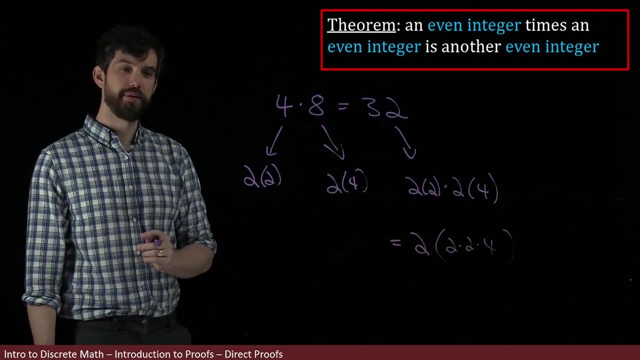 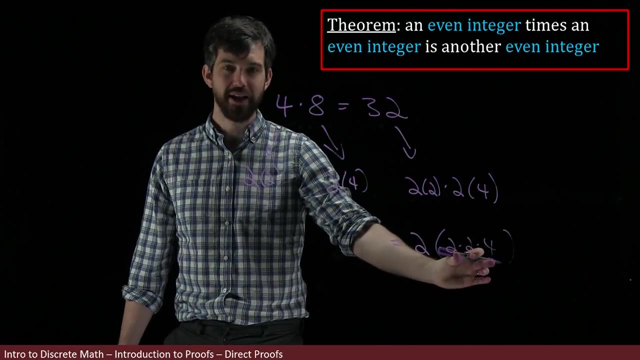 and that's what we want it. for it to be even right, We want it to be two times a bunch of other stuff. This is like two times a bunch of other stuff, In this case, two times two times four. So I think that that works. 32 is an even integer, because it's written as twice times blah And the blah. 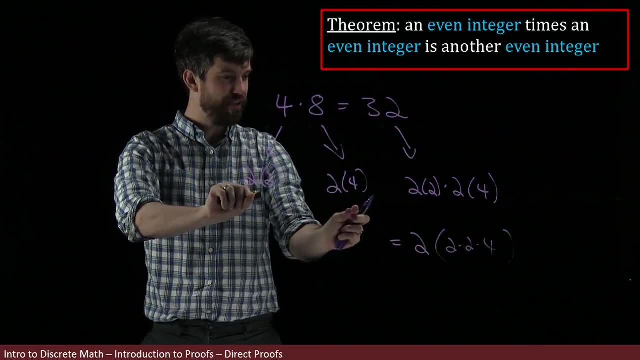 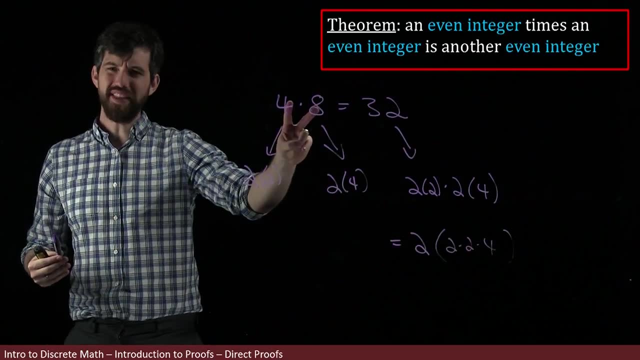 all came about because I sort of broke up my four and eight and I applied their definition and I put them together. So this is sort of my intuitive picture here. I can kind of imagine that the four and the eight don't really matter. It could be any m and n here and I could get any. 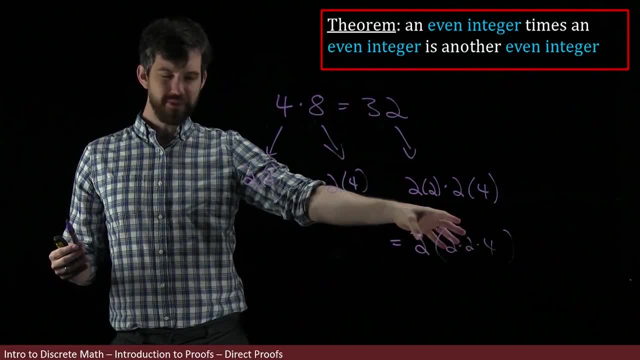 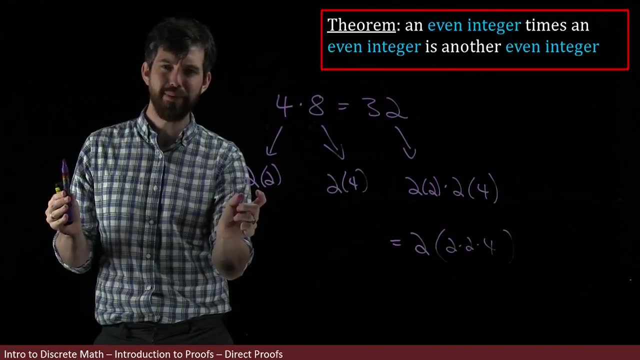 values out of this, And then, when you multiply them together, I think it should work. I'm not 100% sure yet, but I think it should work that you just sort of get the one two that came maybe from the first one, and everything else gets lumped together All right. So that's my tentative, intuitive picture. 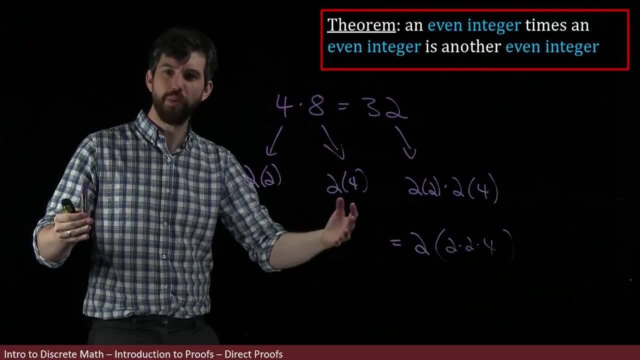 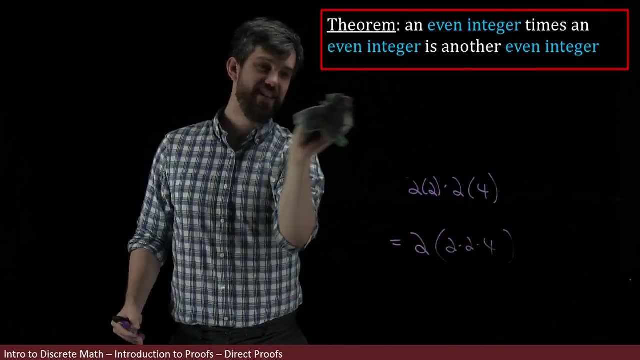 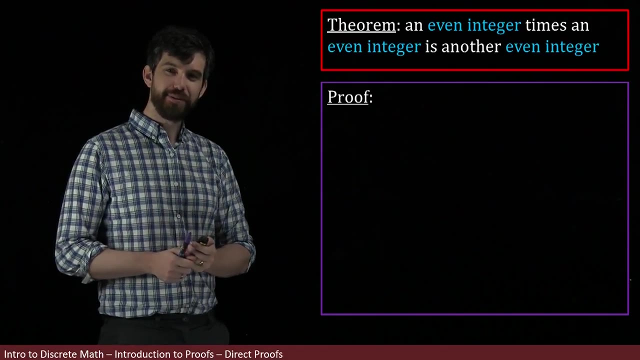 why I think maybe this is going to be an even integer, But let's see whether we can formalize this properly with all of our precise definitions and fill out an actual proof. All right, So here we are, Step four. We're going to be trying to prove this claim And I want to note: 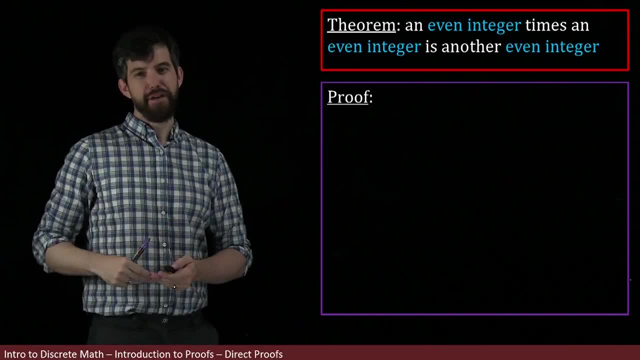 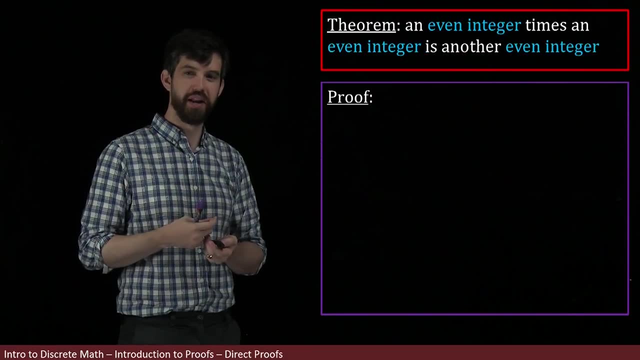 that the proof that we're going to have here is going to fit a relatively standard format. In fact, we don't really necessarily care about this particular theorem, although that's what we're going to use to illustrate the point, But the format is going to be the same as the standard format, So we're going to use the standard. format, But the format is going to be the same as the standard format. So we're going to use the standard format. So we're going to use the standard format. So we're going to use the standard format And it's going to. 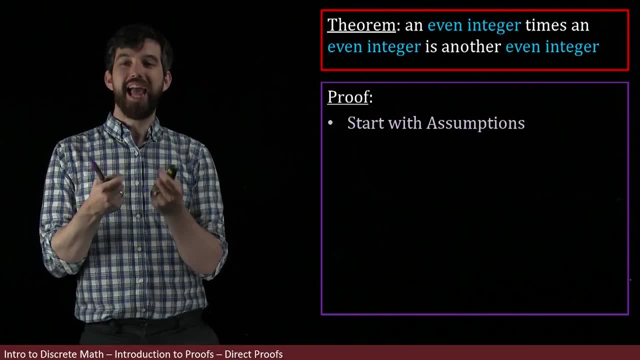 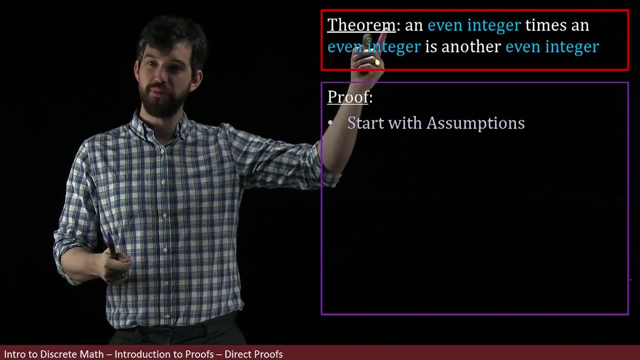 be quite constant. Indeed, one of the first things that we're going to want to do is we want to write down whatever our assumptions are going to be. That's how we're going to start our proof. We say: well, what do we know for sure? In this case, we know that. 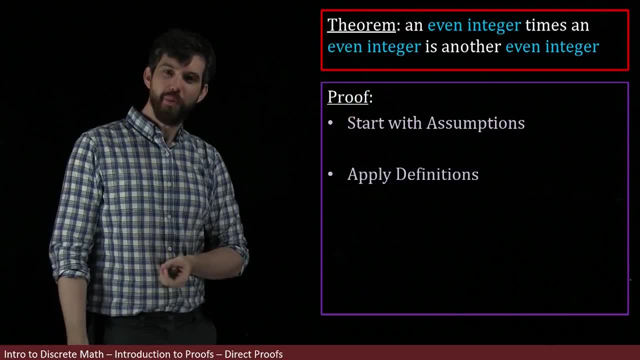 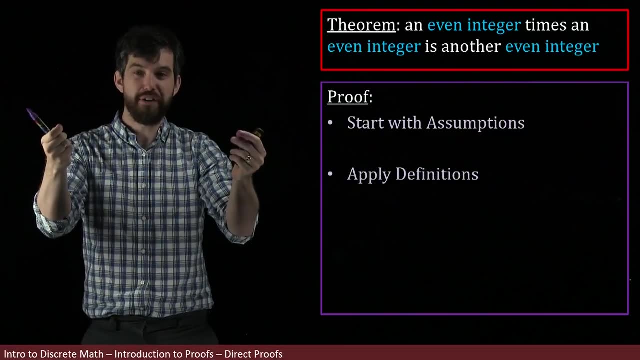 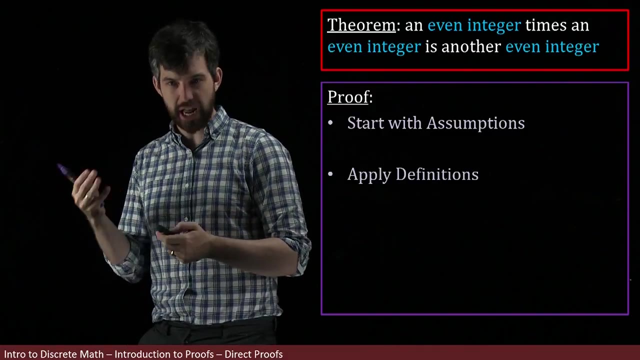 we have two different even integers. That's what we know. And then we want to apply our definitions. OK, you've got two even integers, So what? What does that mean? And we had that really formal definition of what it meant to have two different even integers. And then, in the middle- this is the part that 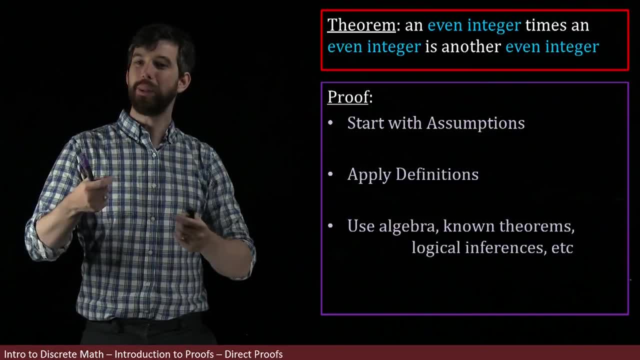 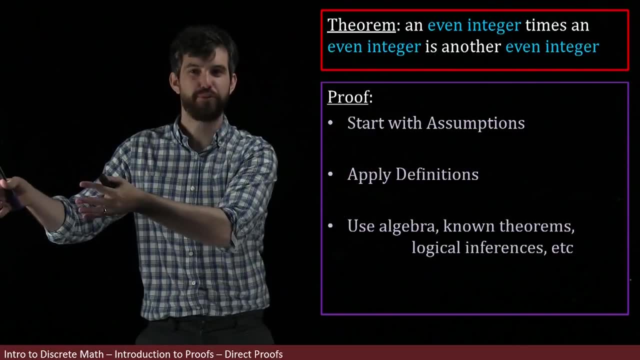 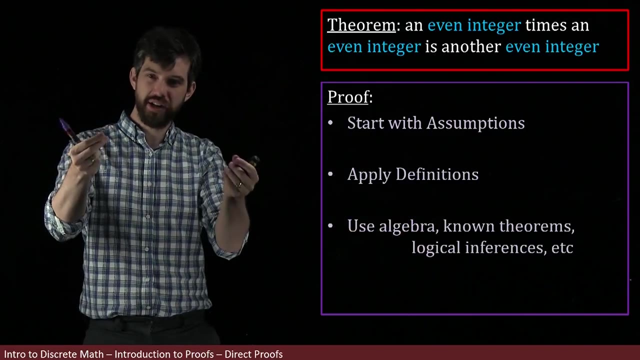 and varies from proof to proof, is we got to do our playing around? this is where we use algebra, where we use logical implications, where we use facts that we've proven previously or that we've looked up somewhere. this is where we do all of our manipulations and we try to take these starting assumptions that have 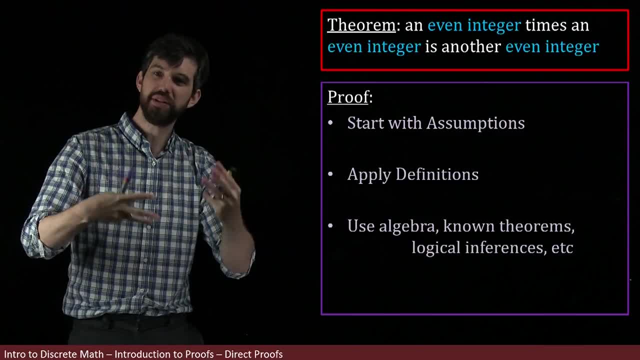 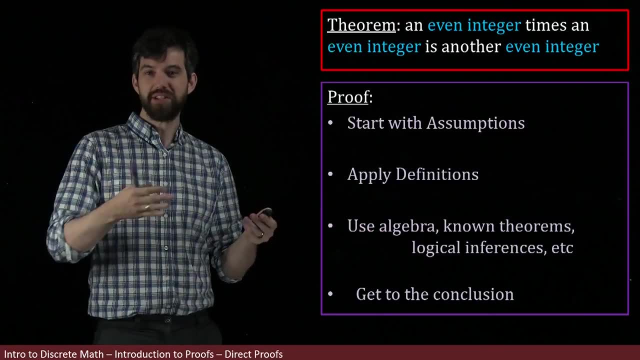 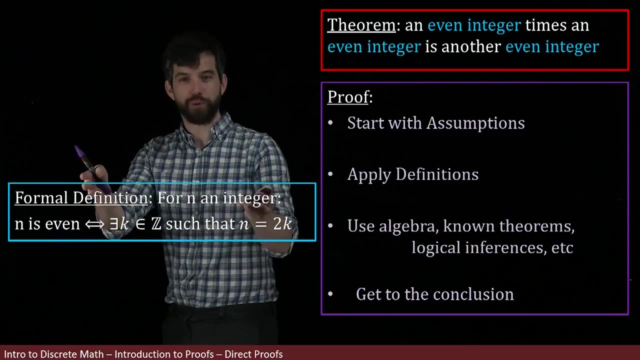 been precisely written with their definitions, and keep on massaging them using all these different tools until it looks like our conclusion. alright, so that's the the basic structure that I'm going to be trying to put in place when I do my proof. I also want to note that I can bring over at any point my formal 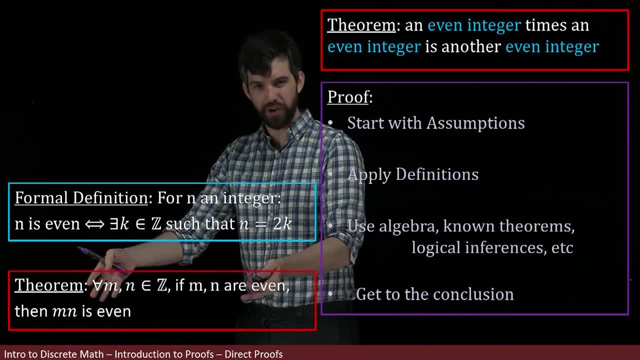 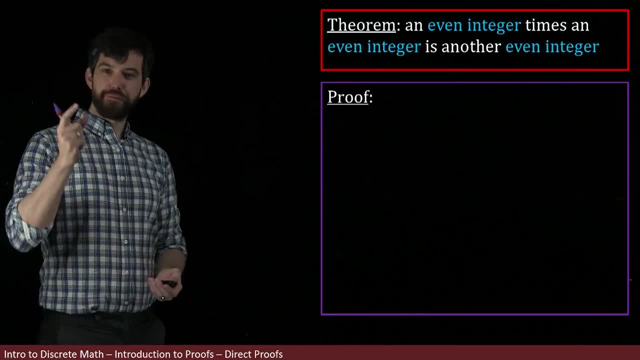 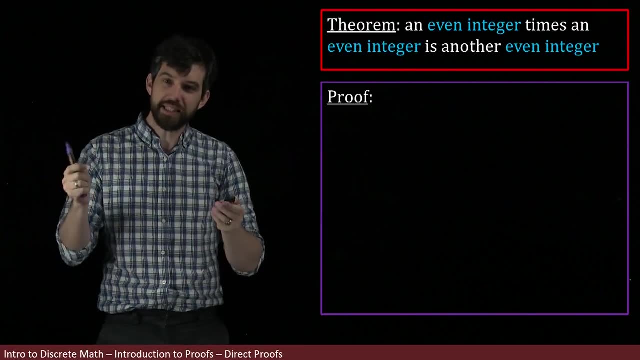 definition, or I could bring over at any point my formal statement of my theorems that I have these here if and when I need them. all right. so first up was to state what our assumptions are going to be in this case. the state of the assumptions is that we are going to begin with M and. 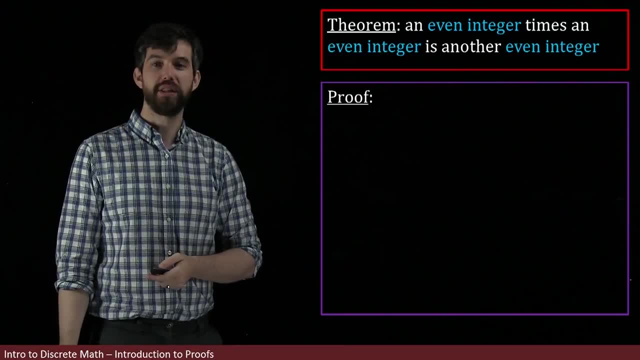 A, and then we're going to begin with A, and then we're going to begin with B, and, and then we're going to begin with A, and then we're going to begin with B and n being an even integer. So this is my first line of my proof. 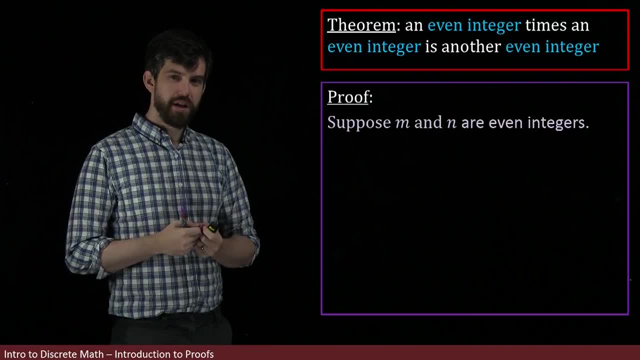 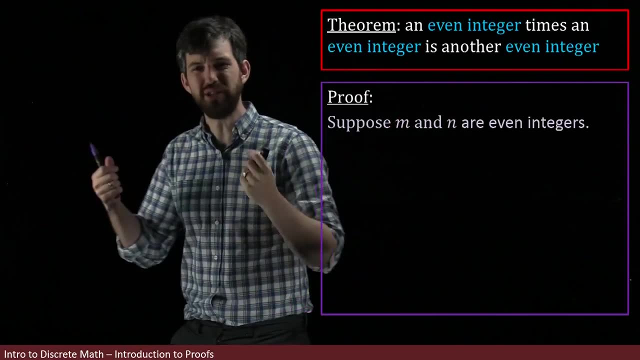 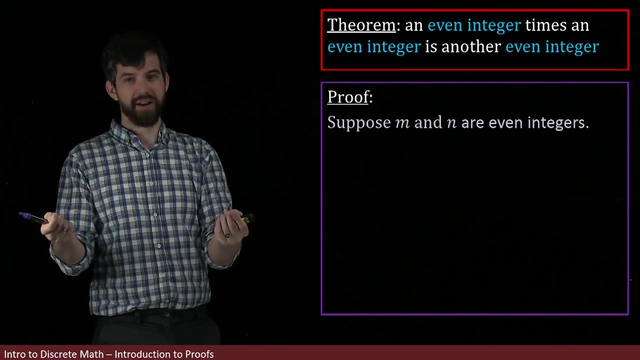 Suppose m and n are even integers. Maybe the one thing I want to note about this line is that this line that I have here- suppose m and n are even integers- is I'm choosing my m and n completely arbitrarily. In fact, this is the same thing as saying: for all m and n. 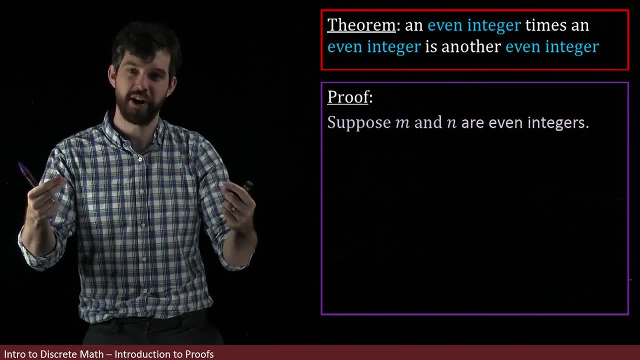 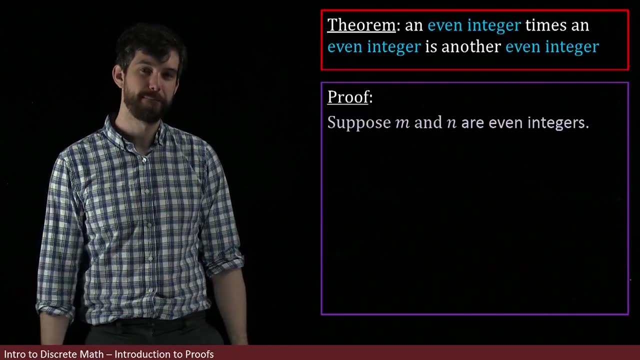 If I just choose any arbitrary pair and prove it for an arbitrary pair, I've proved it for everything. So that's what I'm doing. I'm supposing that I've got two even integers and I'm giving them some labels: m and n. 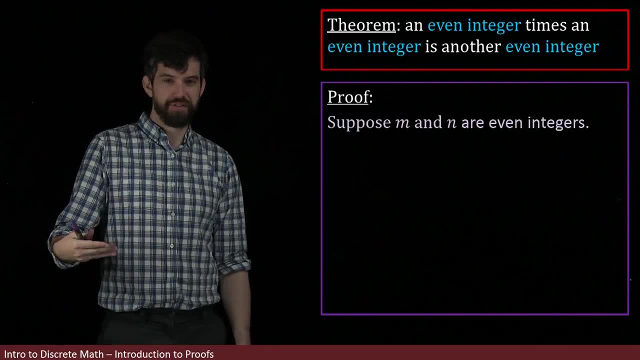 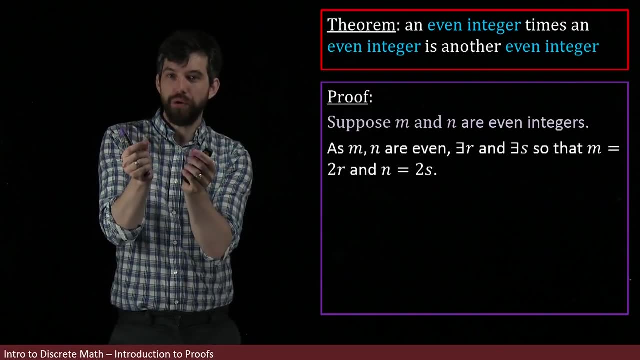 Now, next up, we want to figure out how we apply our definition. So even integers meant specific things. So in this case, because they are both even, it meant that we got two other numbers, and I'm going to call these other numbers: r and s. 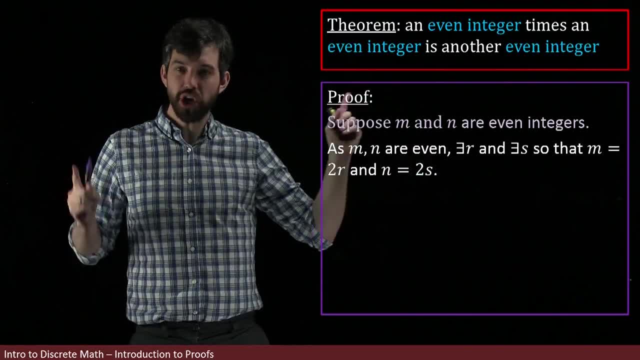 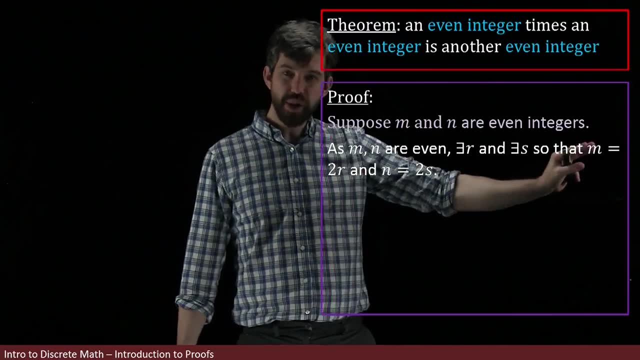 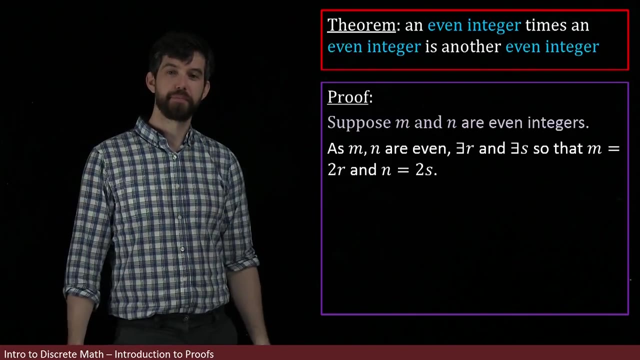 So I'm going to say that there exists an r and an s, so that the m is twice r and the n is twice s. So this statement here is me applying my definition of an even integer to the two even integers that I have, the m and the n. 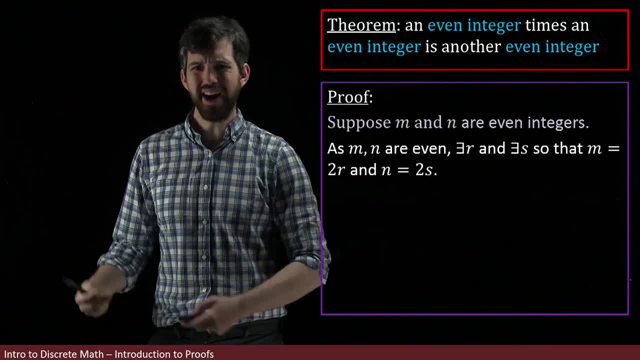 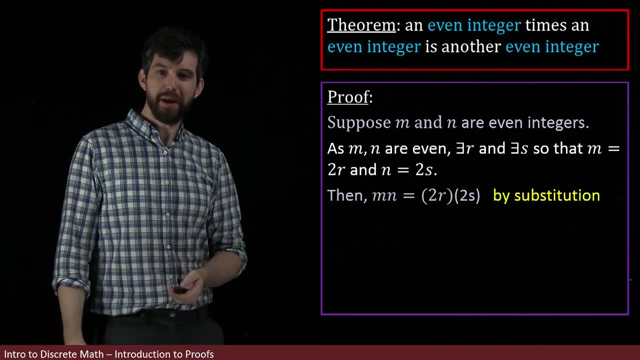 Next up, I want to do some algebraic manipulations. We're trying to get to m times n right, That's what our goal is, And we want to show that m times n is an even integer. So maybe my first step is just to say: 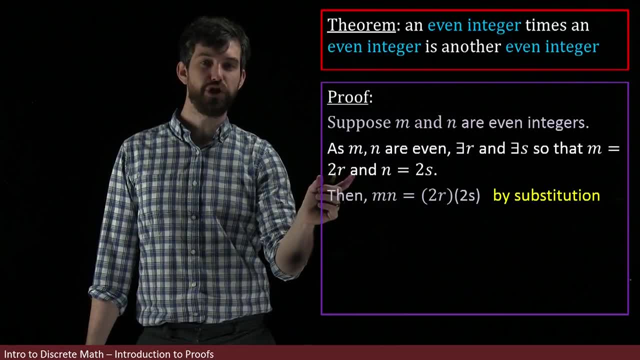 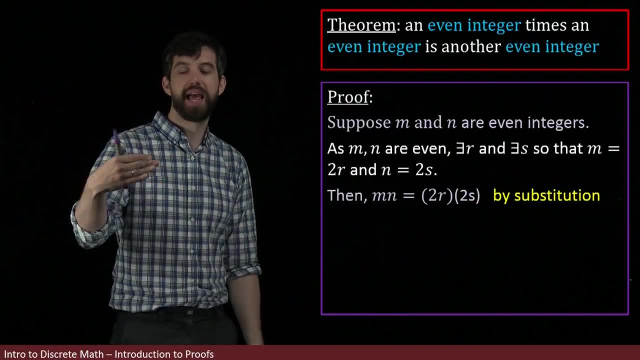 well, look, I've got my m times n. Let's substitute in the two r and the two s that I have for the m and the n, and I can write it down this way. So I've substituted in the values that I have for my definition. 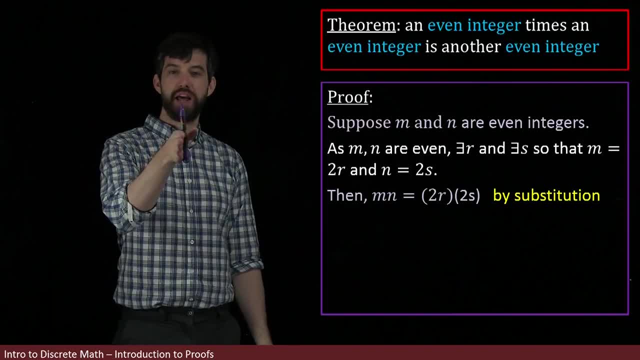 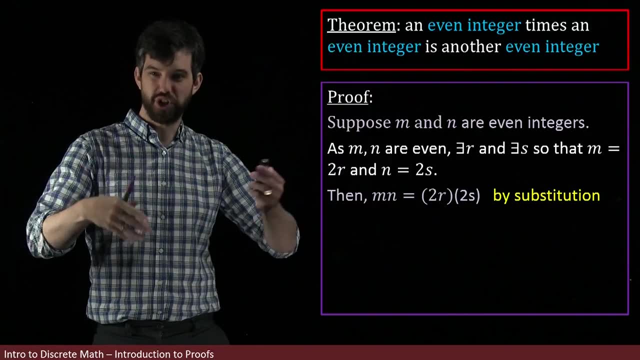 I've related m and n to twice r times twice s. Next up is the little bit of algebraic manipulation that we saw previously, when we were just sort of playing around and seeing what might be true. I've got one 2 inside of here. 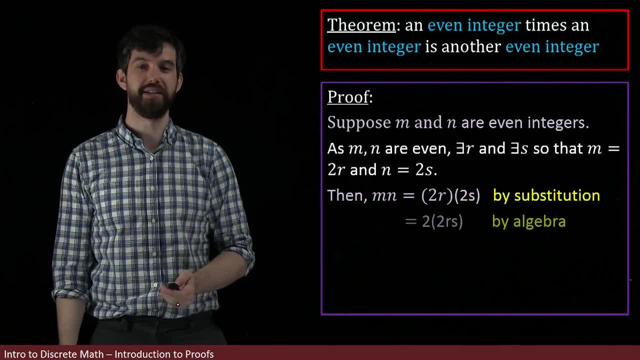 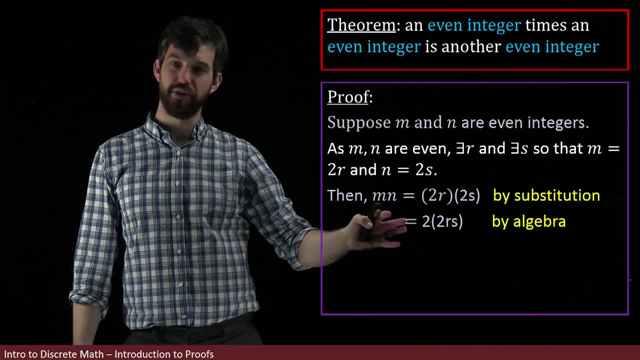 So let's pull that out the front and just leave everything else sort of hanging behind it. So I'm writing this as 2 of 2rs. This property, by the way, is referred to as associativity. I also move one of the 2s around. 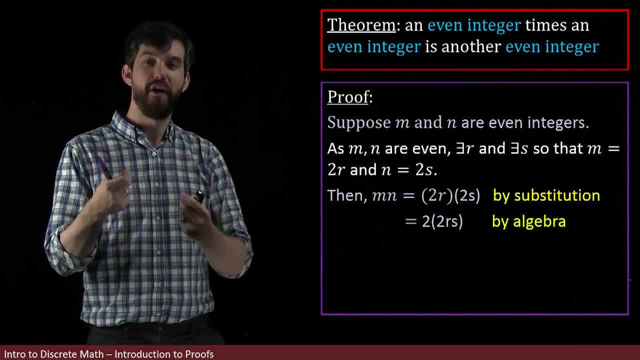 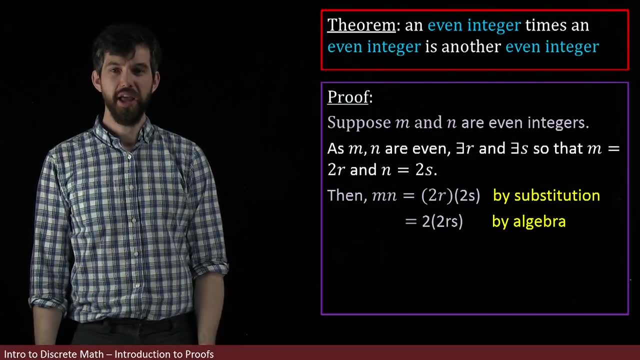 But these are properties that we know to be true from numbers, that we can change our brackets around and we can reorder things. That's perfectly fine, All right. so what have we got? We've got that the m times n is indeed going to be written. 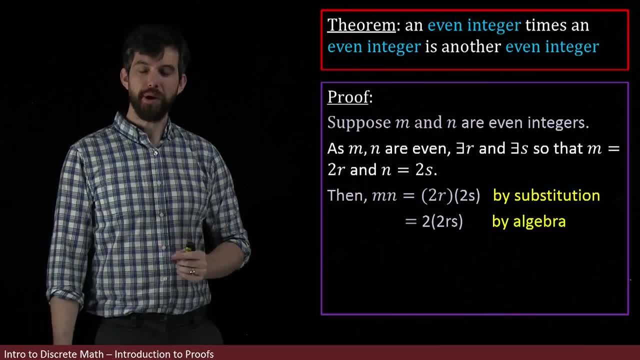 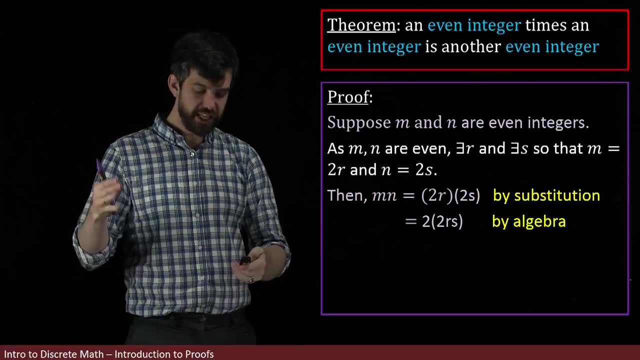 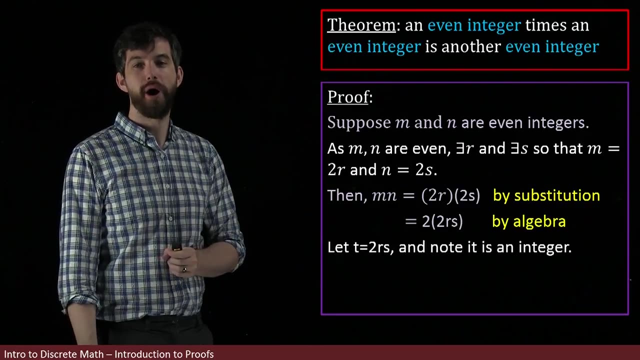 as twice something. But I need to really lock out my little proof here that twice something, the something should be given a specific name and noted that it is an integer. So that's what I'm going to do. next, I'm going to say: let t equal the 2rs. 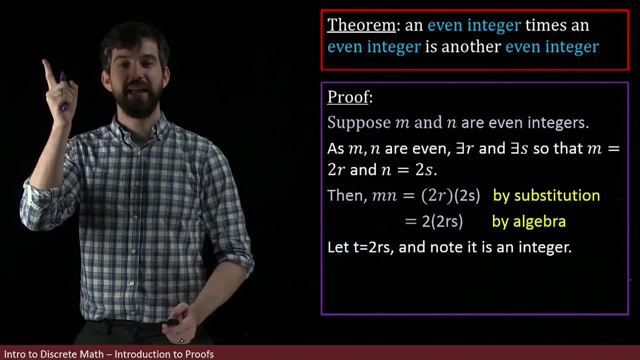 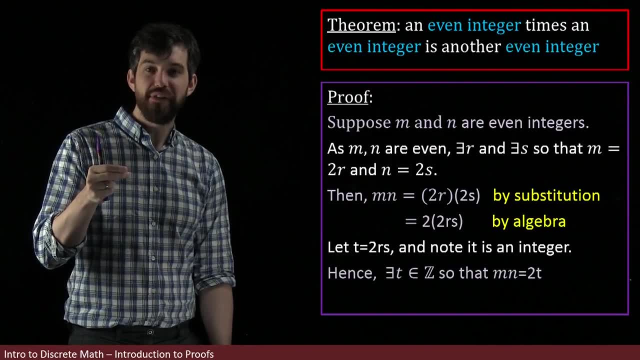 Letting all this stuff over here be given a name And it is an integer, And the reason why this is important is that the t that we have that was our existence claim. Remember when we talked about our definition of it being an even integer. 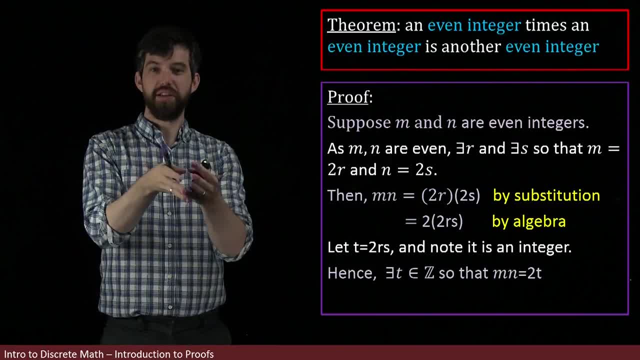 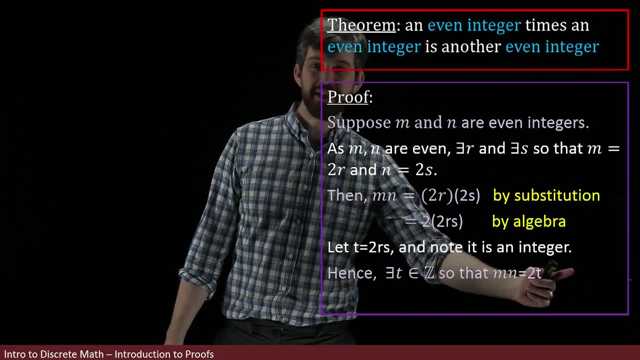 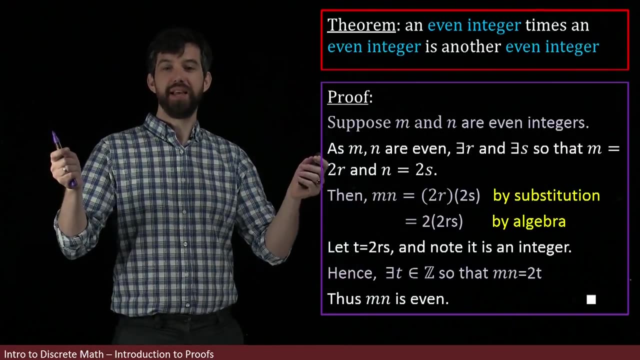 There existed something in the integers so that whatever you had was twice it. That's precisely that statement. There exists a t so that the product is twice that, And the definition of this is that my mn is an even integer. And so I write thus: mn is an even integer. 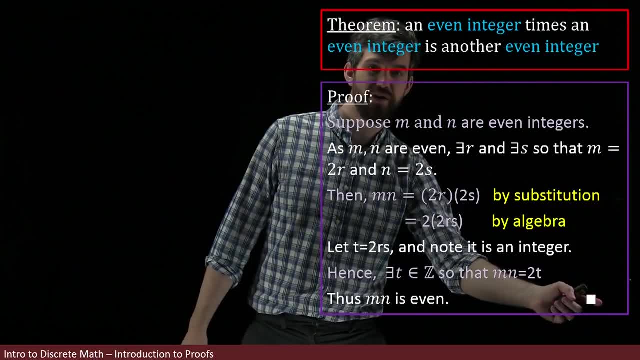 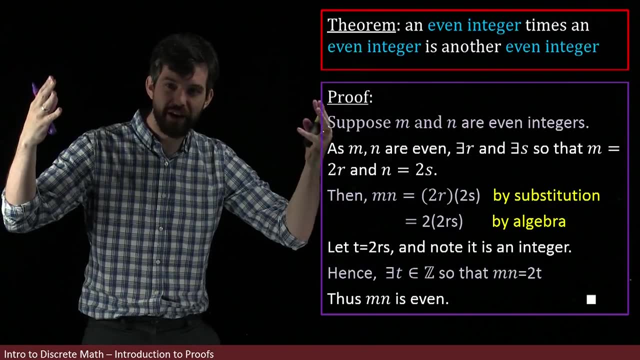 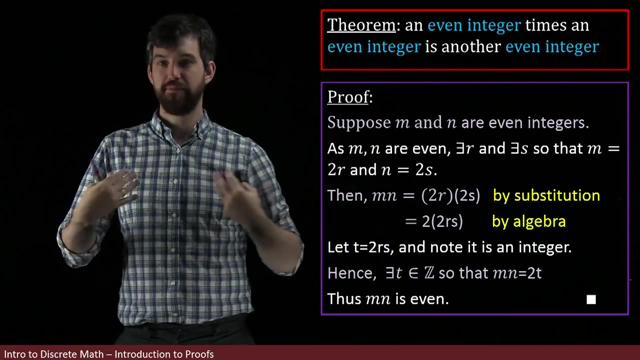 And then I finish off my proof by putting this little square symbol here that stands for QED. We put that at the end of our proofs to be like: voila, we have successfully proven what we set out to prove Now In this formal proof, which I believe is convincing. 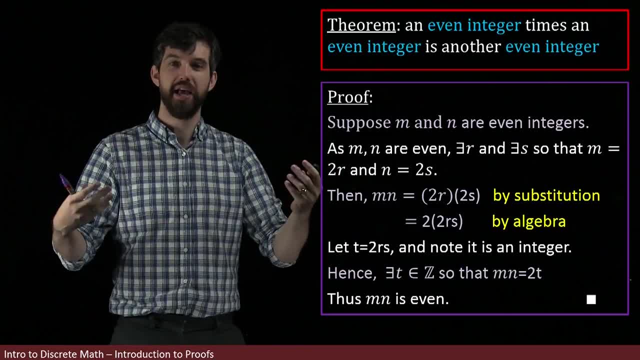 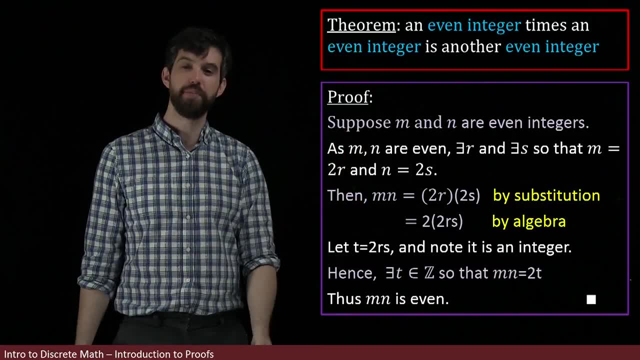 and now that people read this, they can apply it and agree that, yes, indeed, the product to even integers is an even integer, And this structure that we have has a couple different key components that I want to identify. First, I want you to look at the first and last lines. 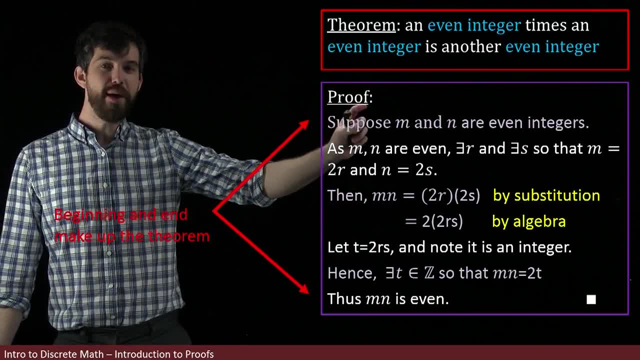 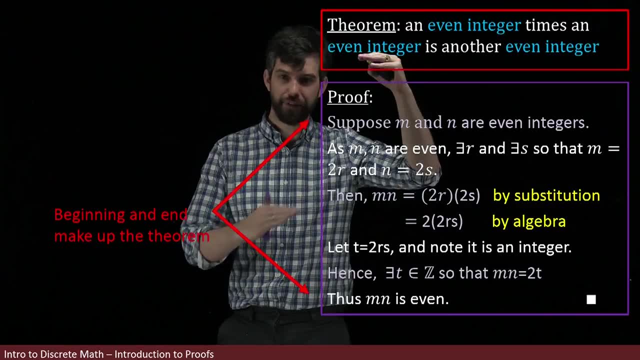 Well notice, if I read them together. Suppose m and n are an even integer, Thus m times n is even. So, in other words, what I have by reading them together- reading the first and the last lines together- is the statement of my theorem. 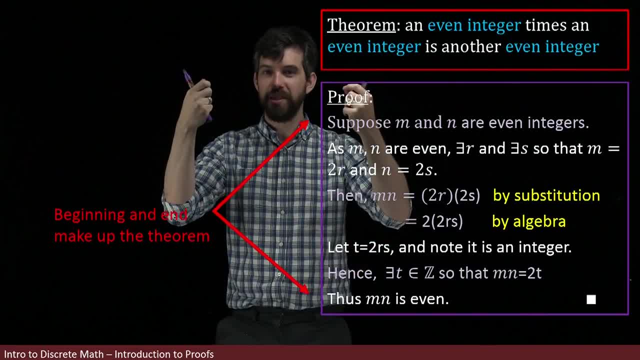 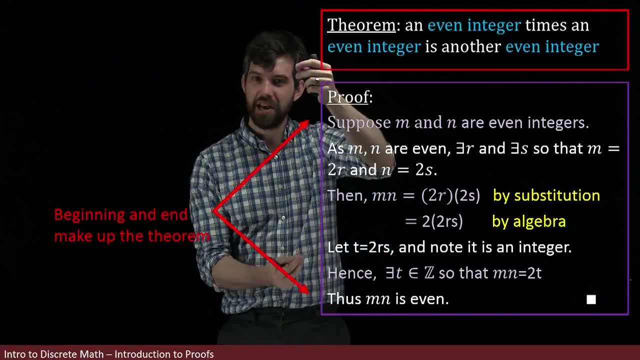 And that's the way that it's supposed to work. You start by assuming the p of x and you get out the q of x. You start by your assumption and you get your conclusion. And then, if you read the beginning and end, 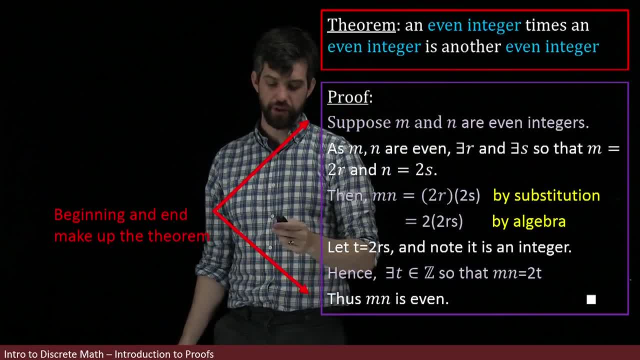 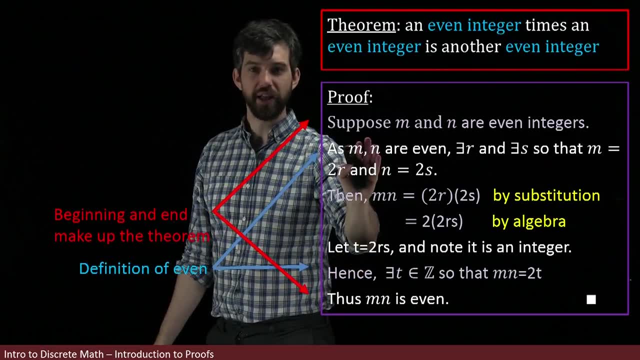 of your proof together. it should be the statement of your theorem, All right. next up, I want to talk about definitions. We use this a couple times. Notice that the first one is right here in the second line And down in the second to last line. 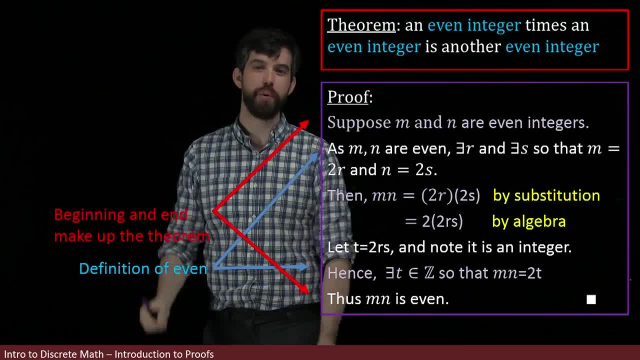 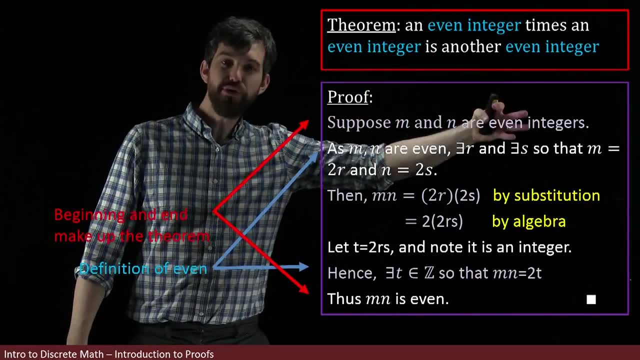 I'm taking the formal definition of even and I'm applying it at both ends. And it makes sense that I'm applying it at both ends because in my statement I begin with a claim about two even integers And then I deduce a claim about even integers. 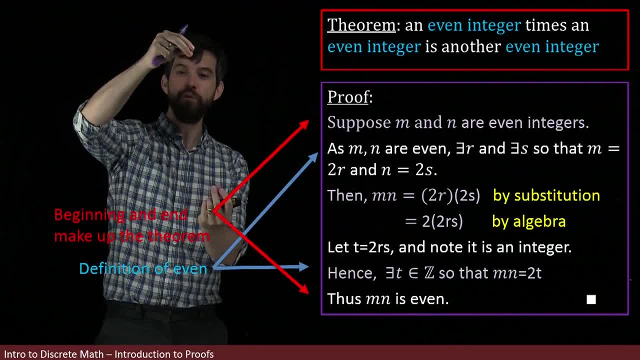 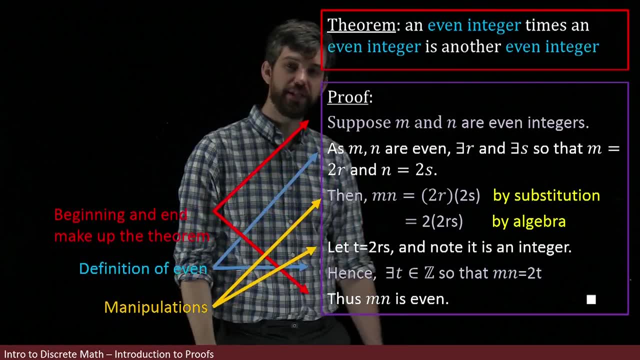 So if I split that up to the start of the beginning, I sort of go in one level of applying the definitions right at the beginning and right before the end, And then the stuff in the middle. here this is going to be my manipulations. 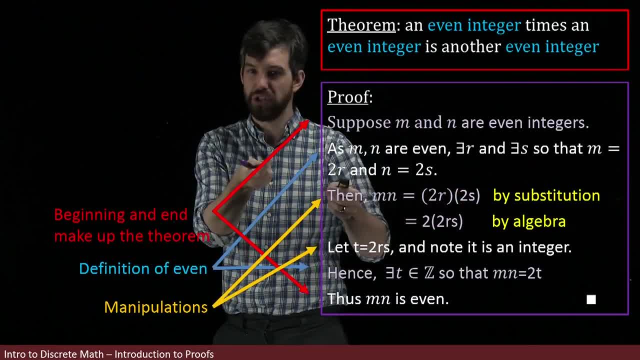 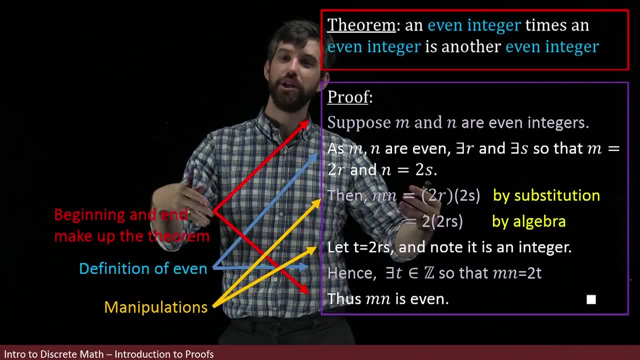 And this, in general, could be all sorts of different things. In this case, I have a little substitution, a little bit of associativity, a little bit of algebra to manipulate what I had in my assumptions into a form that looked like my conclusions. 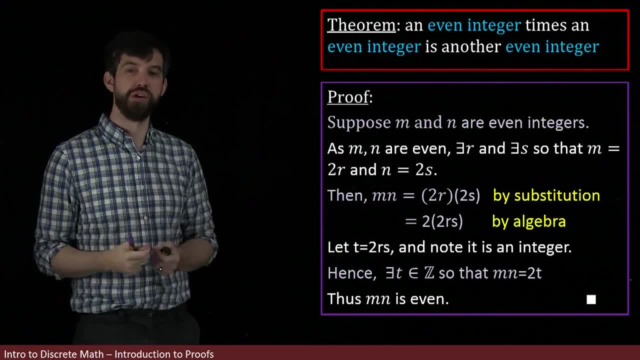 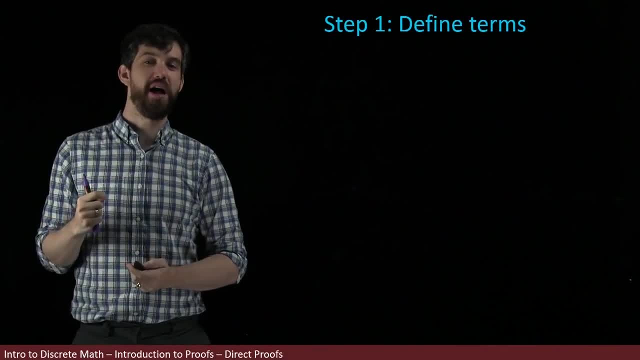 So this is the general strategy that I use when trying to prove things, And maybe we can summarize it like this: Step one: define our terms. That's what we did. We defined our even terms. Step two: state our theorem formally, so we know exactly what it is that we're trying to say. 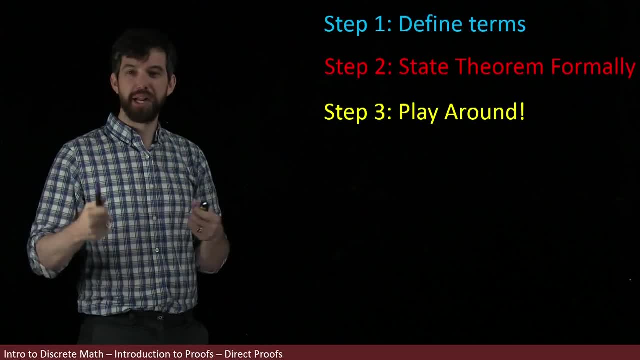 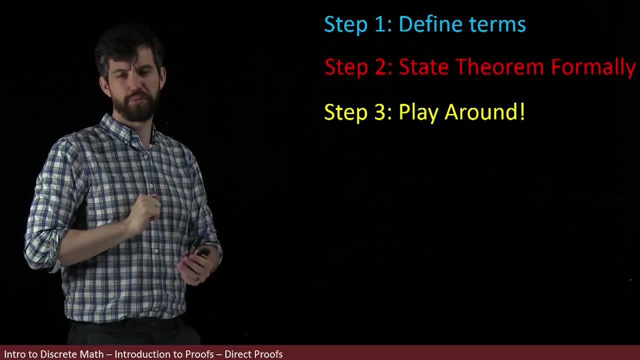 Then this is the most important part. step three: This is my playing around. This is me trying to figure out. how do I know this theorem is true? What's the key step? What am I going to put into my formal proof? 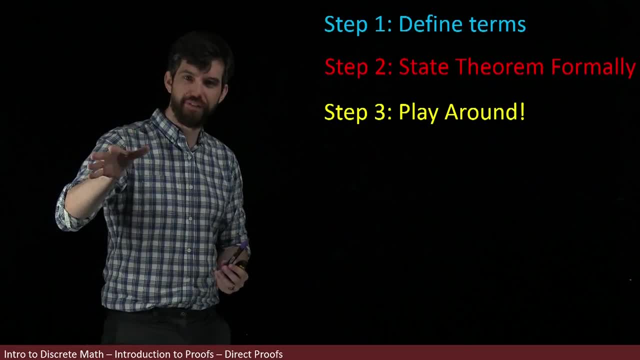 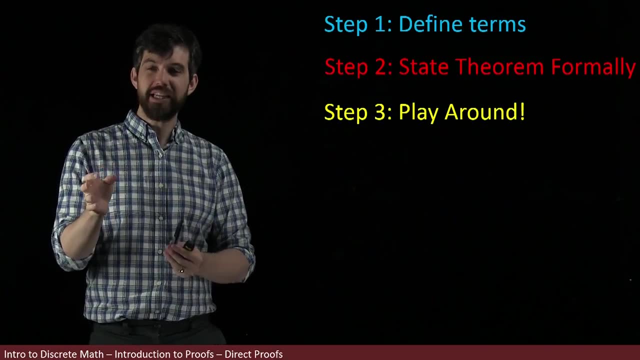 By the way, you could do step three even earlier than this. Maybe you don't want to formally define things. You want to do your playing around ahead of time. That's also OK, Although I will caution. it's often helpful, at least when we're starting out here. 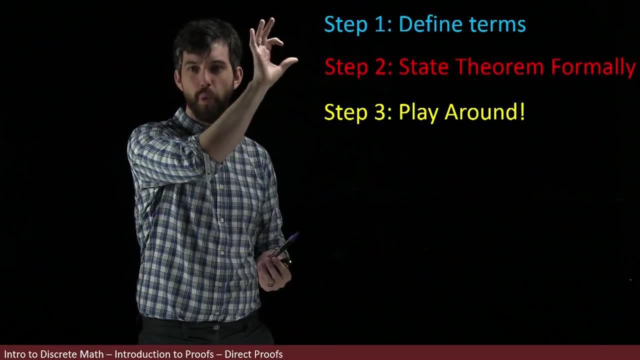 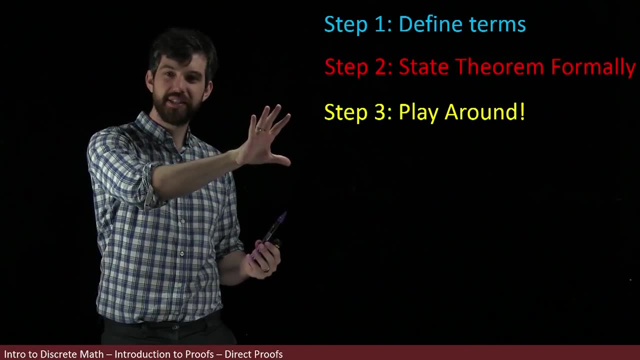 to go through this process of really formally defining what it is that I'm trying to state. That will help inform my playing around. But if you want to do some playing around at the beginning and then some precise statements, then maybe a little bit more playing around. knock yourself out.